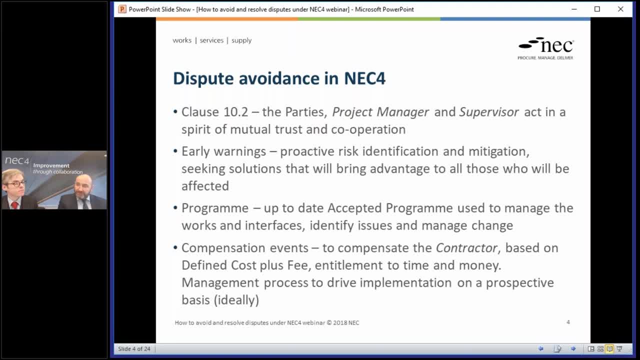 So there's a requirement here for the parties to be, if you like, fair and reasonable, to try and work together to reduce or mitigate the effect of events that could turn into disputes, or to be perhaps more reasonable in trying to agree how those disputes are. 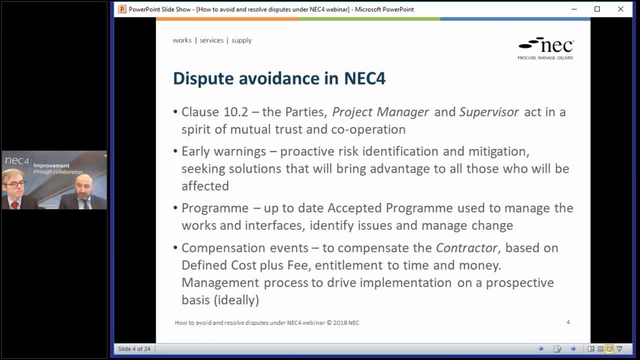 dealt with and resolved, albeit they're always governed by the actual rules of the contract. They have to comply with what the contract says. Another big thing we have in the contract is early warnings. Early warnings is a proactive risk identification and mitigation tool, The idea being that either party can raise an 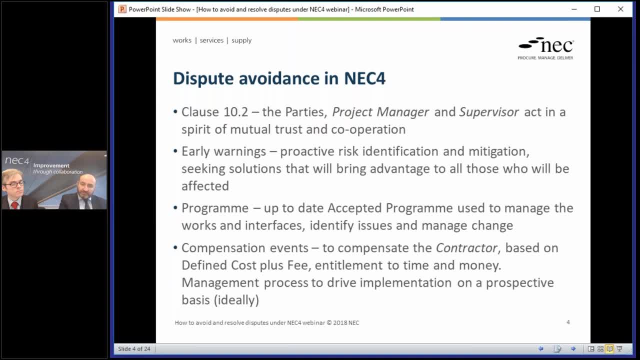 early warning of an event which they think will affect time, cost or quality. And that's regardless of who's liable, who's responsible, whether it will or will not become a compensation event. The idea being that, regardless of cause or liability, you raise the issue, you deal. 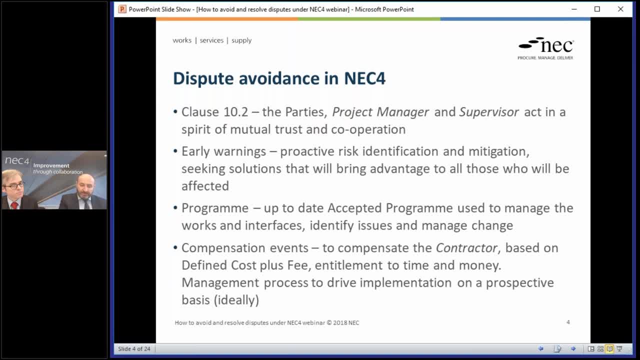 with it as quickly as possible in a way that brings advantage to all those affected, So there's less likely to be a cost or delay flowing from it that could then become the source of a dispute, So try and keep that in mind. The second thing we have in the contract is early warning. Early warning is a very important 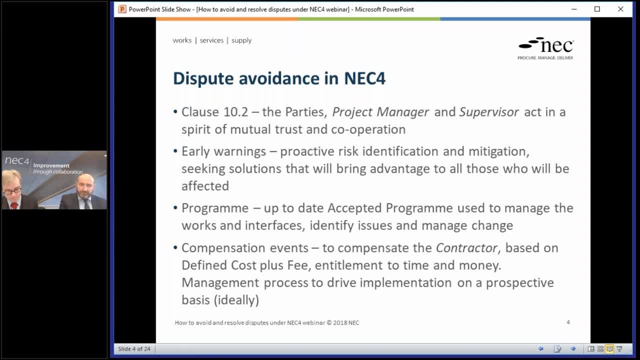 part of any NEC contract, very much at the heart of the contracts, And we have this concept of the accepted program And that should be used to do two things, especially to manage the works. So, looking at interfaces between this contract and other contracts, agreeing 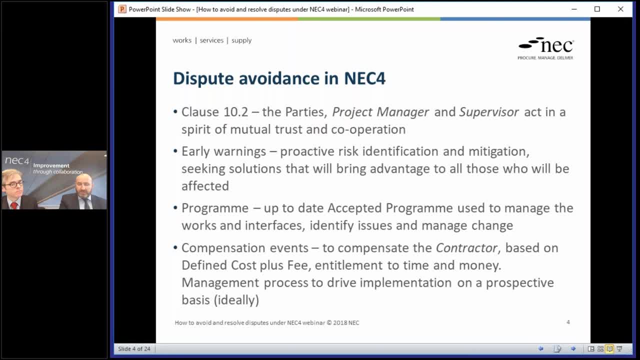 when the client or others will do certain activities. So the parties have clarity over when they have to do it, When they have to do things, what they've committed to do, and by when. So that should mean there's less problems, there's less issues that flow from that. People know what they're. 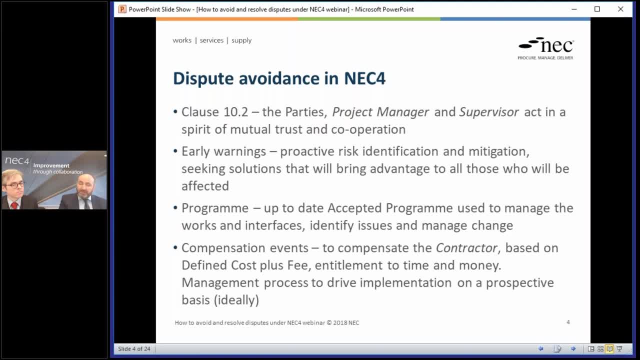 meant to do and therefore they can hopefully deliver to that. That's less likely to cause delays and problems And also the accepted program is used to manage change. I'm really linking with the final point on the slide: compensation events. We have a process in 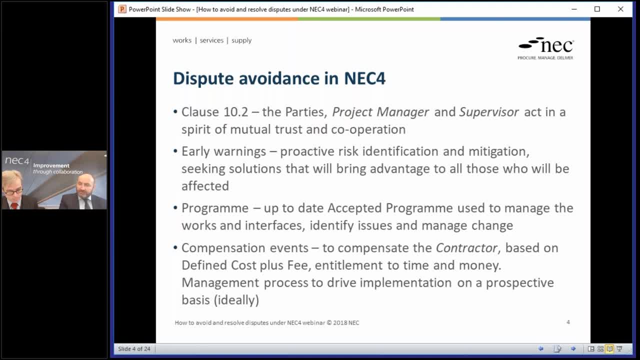 the contract to try and work out the time and cost effects of change as and when it occurs- Hopefully ahead of it occurring, where possible on a prospective basis. And this is trying to encourage the parties to use this up to date accepted program to impact delay events. 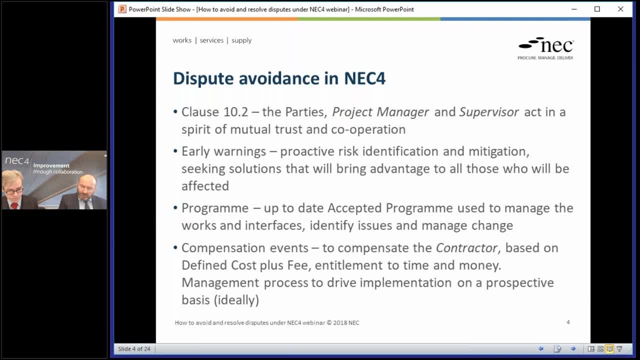 to look at the effect of defined cost plus fee, So what the cost really will be to the contractor for the change. So the contractor will be compensated for the event because it's not their risk under the contract. They should recover a fair entitlement in accordance with the provisions of the contract And that again. 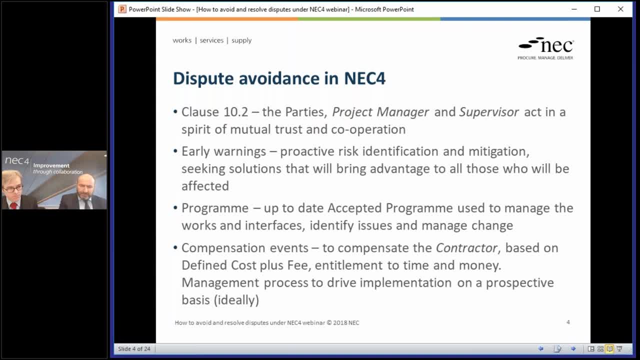 should remove the potential for claims. We don't have gamesmanship around bill rates being used or rates in a tender that could be seen to be disproportionately high or low. The idea is we're compensating the contractor and I think that's most importantly of all. we have some very clear time scales for that process. 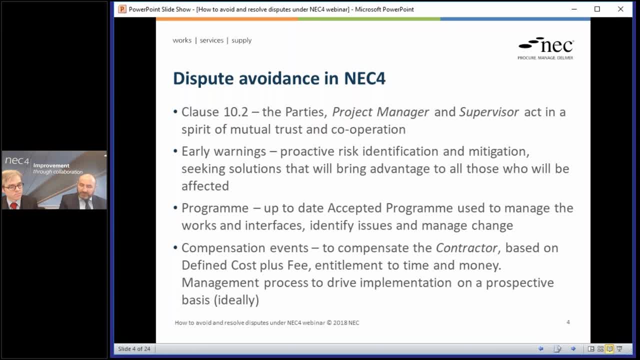 and ways of either party to drive the compensation process to a conclusion. So that allows the parties to you know, hopefully agree things as and when they occur, or at least a decision is taken as and when things occur, that is closed out, finalized and we move on rather than it drift. 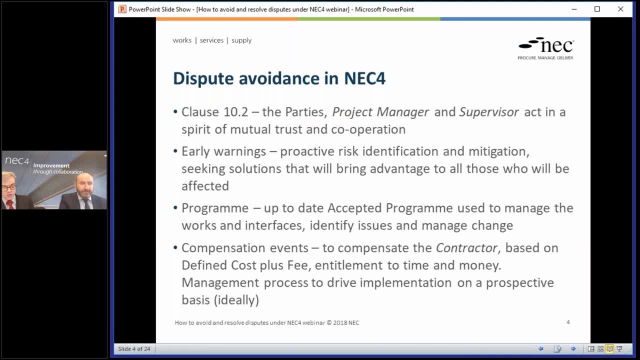 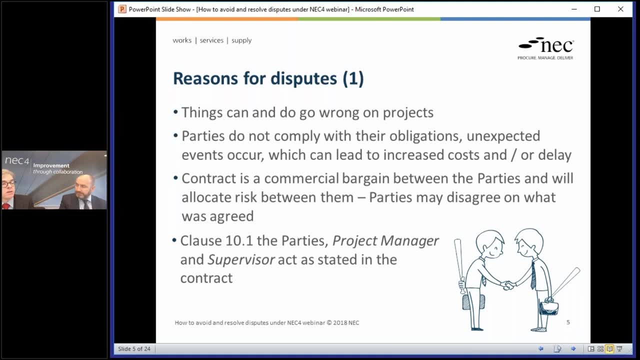 fester and become a much bigger issue. So that's right, I mean. so the dispute avoidance part is a very big part because I mean most of these disputes they just go away. those mechanisms are there, the compensation event mechanism, particularly to make the disputes go away. but let's not be. 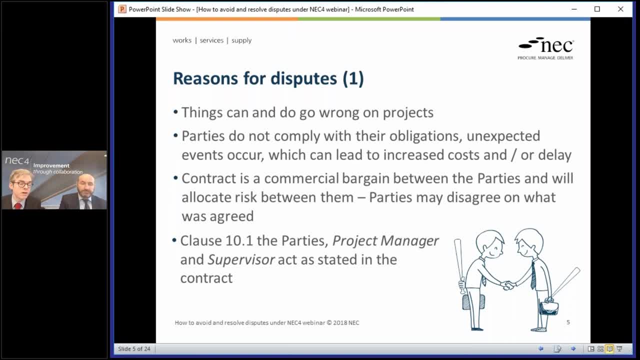 naive. I mean, there are disputes that happen irrespective of those mechanisms and you know things go wrong, as we all know. The first problem that occurs really is that unexpected things happen: ground condition problems, weather problems, third-party interventions. these can lead to increased costs and delay, which usually bears on the contractor in the first. 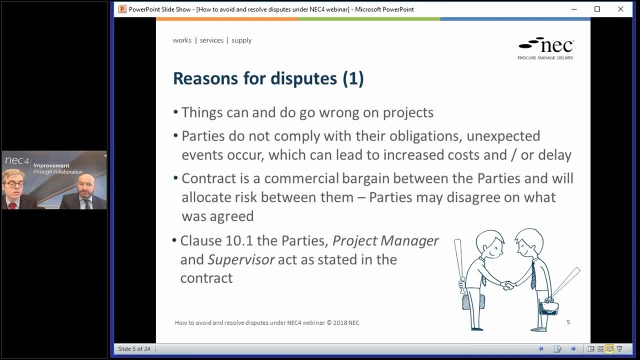 instance, but there's usually going to be some sort of discussion, or which can lead to a dispute, about who ultimately carries it, whether it's the contractor or the employer, and, of course, when you're talking about a dispute, that the first place one goes really is the contract, as 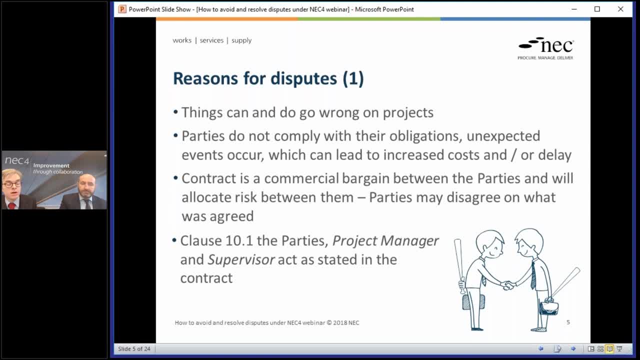 a primary mechanism of dealing with your dispute, and the NEC is founded on the basic concept that the contract's a commercial bargain and, as recognized in English law and most of the systems of law around the world, the idea of the contract is to allocate risk that you know there are risk. 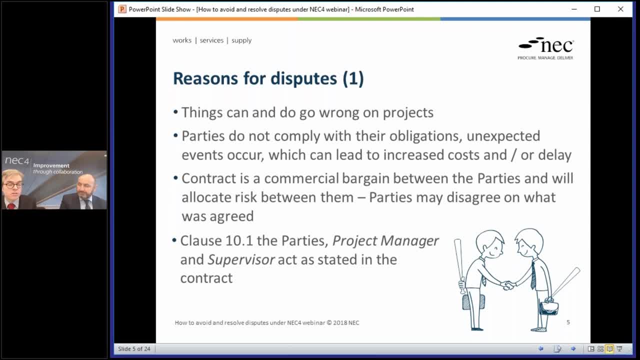 events. things will occur, and we must allocate risk, and the parties have already done that in their contract, and so we don't just have 10.2. it's not as if the parties are just asking for 10.2. it's not as if the parties are just asking for 10.2. it's not as if the parties are. 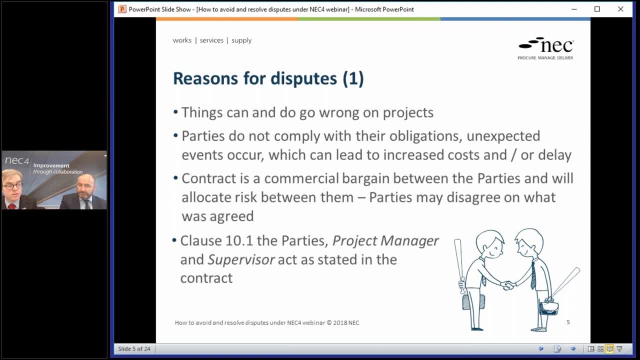 just asking for 10.2. it's not as if the parties are just asking, acting in a spirit of cooperation. there's also the rule in 10.1 that the parties, the PM and the supervisor all have to act in accordance with the contract, and so that's the primary approach to dealing with disputes. 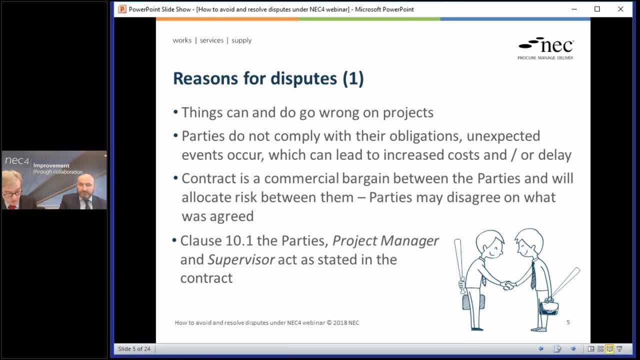 is that the parties are obliged to act in accordance with their contract. yeah, and I think that's a really important point to make, that we do have this idea 10.1. that is the prime obligation in the contract. the parties have to do what the contract says. as you've already stated there, the 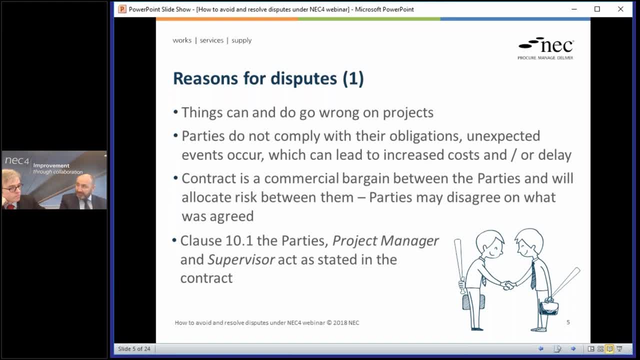 contract is this commercial bargain that the parties have signed up to. there is an allocation of risk, and so certain events will occur for which the contractor may be compensated, and some for which they won't be compensated. so there may be times when a party has to pay out money, or does. 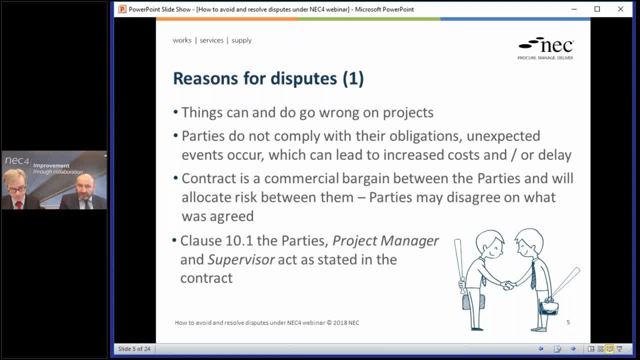 not receive money and that can leave a sour taste, it can cause ill feeling. but ultimately you have to operate the contract as written. you can't just ignore that commercial bargain, the rules of the contract and just you know. try to agree everything. you have to operate the contract. 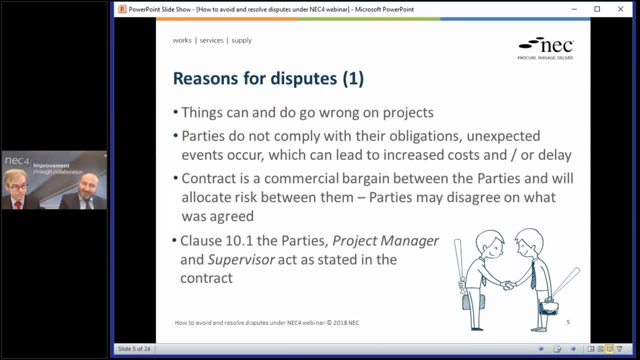 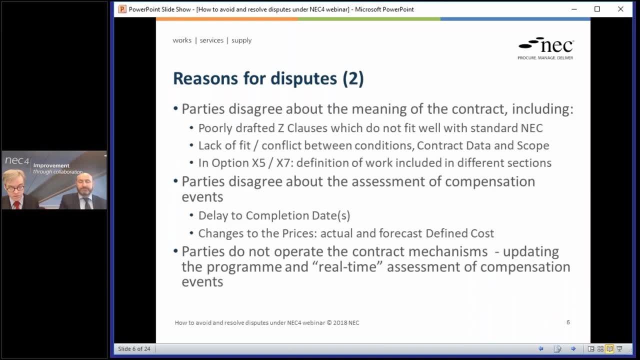 as written, but not forgetting 10.2, in the right spirit, that spirit of mutual trust and cooperation, and that's right and in most cases so in most cases, the disputes go away because of the avoidance mechanisms. there's another large category of disputes that will go away simply because the 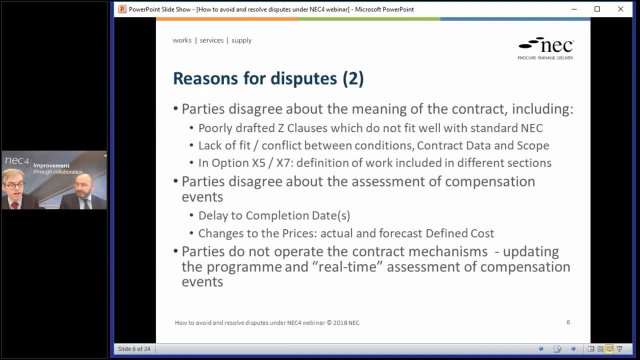 contract deals with it. it's quite clear who's responsible for that or for that, and really what you're dealing with after that is a rump of disputes, where it isn't avoided and the parties can't agree on the words there are frequently. I'm just talking about disputes we've had recently under the NEC suite. 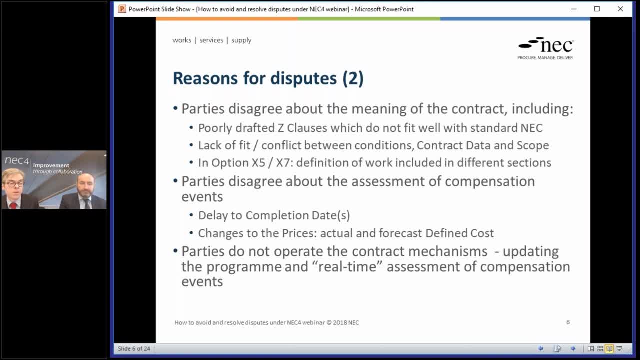 parties can disagree about the meaning of the words in the contract. that doesn't happen so much with the standard terms, but what does happen is that parties will often have zed clauses, bespoke clauses that they like to have in there, and those zed clauses might be well drafted in themselves. 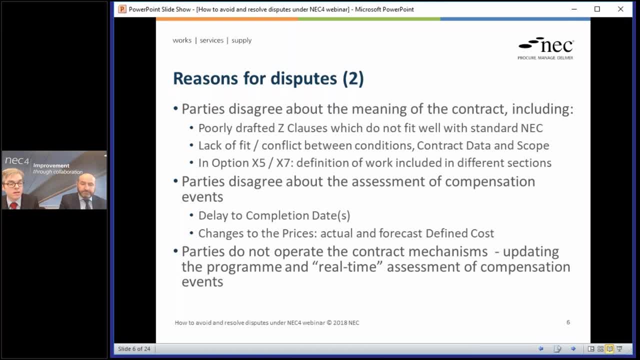 and might work well in other contracts, but they might not fit well with the mechanisms of how standard NEC work. but they might work well in other contracts, but they might not fit well with the mechanisms of how standard NEC work works, particularly in relation to assessment of events and allocation of risks. another problem: 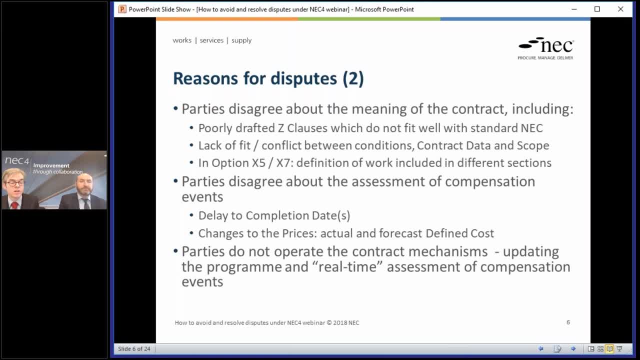 you have is that there's different sections of the contract. you have the main conditions at the front end, the contract data, which has the employers part and the contractors part, and then you have the scope, which, under any of these three, was works information, and we've seen cases where there's 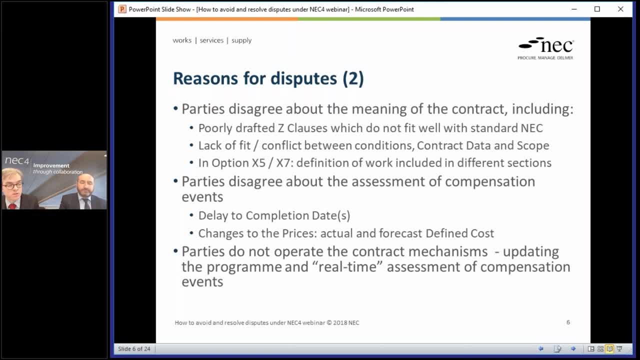 language in those three parts which don't fit together very well. that can lead to disputes, and the final example we've cited there is the final example we've cited there is defining the work. when people divide work into sectional completions, as in the options x5 and x7, there's frequently a discussion about precisely what work. 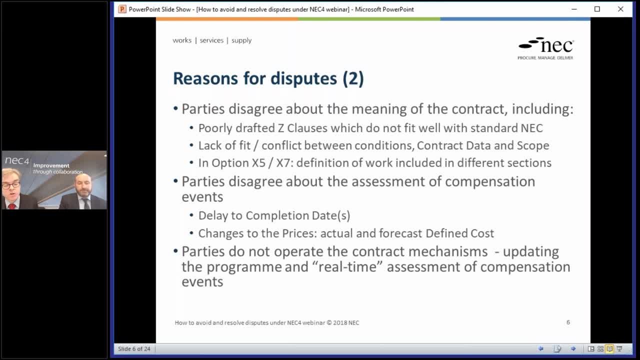 was in, was in what section? disagreements also about the assessment of compensation events. this isn't a. this isn't really a legal point, purely it's about you know what is this compensation event worth, particularly prolongation cost claims quantity surveyors need to come in assess the. 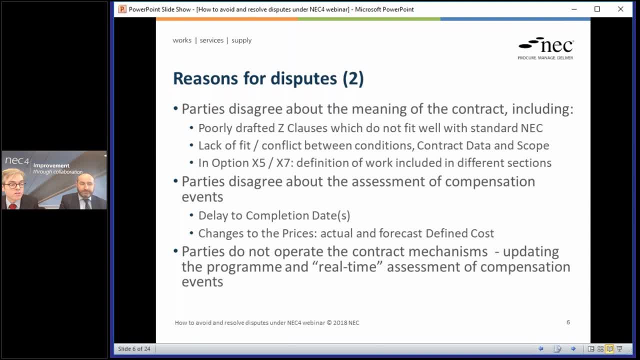 delay. see what the run rate of of cost is and there will be disagreement about that. it's a technical dispute and finally, you know the reasons for disputes that we see is people failing to operate the contract mechanisms. NEC is particularly dependent on applying the correct level of 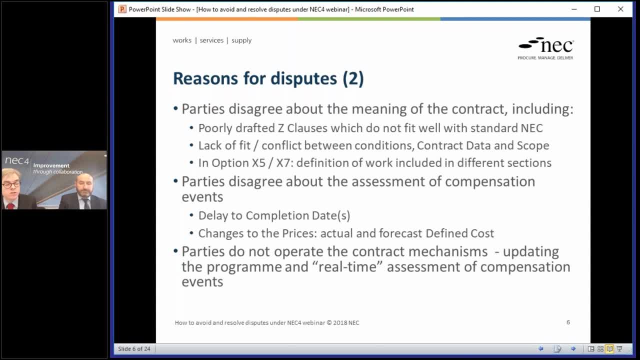 commercial management resource during the running of the contract, during the construction phase, to update the program, which is a key dispute avoidance mechanism, and doing assessment of compensation events as they happen before other things have changed so that you can isolate the effects and people don't do that and 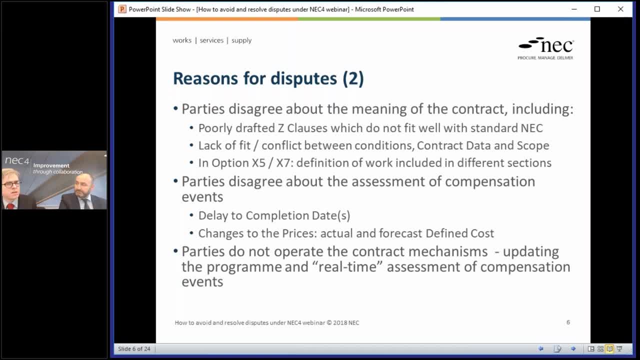 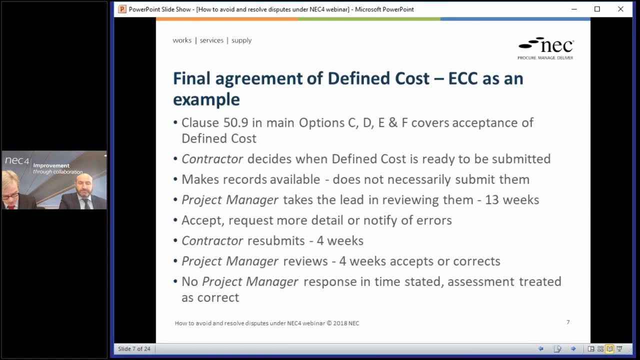 there is a problem of of leaving things to later. there's a problem of not assessing and of not therefore getting any getting any agreement as to who's assumed the risk of a particular event until later in the piece. but we've introduced some, some changes to the suite, I think, here now to do to speed. 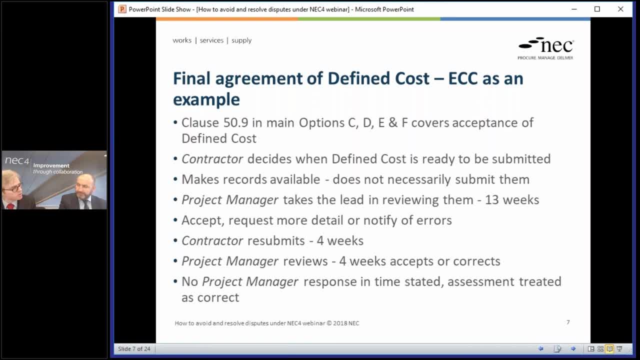 up that process and to oblige parties to get that final resolution. yeah, that's right. within NEC4, we've brought in a couple of provisions to deal with final assessments, the idea being, as you've outlined already, that you know the processes in the contract should lead people to agree things. 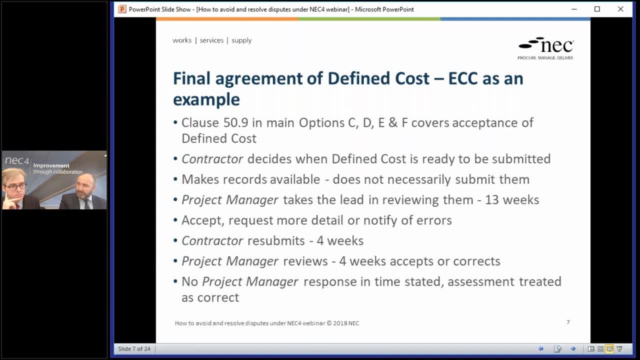 as and when, that there are processes to follow to close out compensation events, etc. however, we still saw in NEC3 issues where things weren't being closed out. people were agreeing to disagree and then things would drift on for a considerable period of time and then other events would impact upon it and things weren't being closed out. so the 1st we've 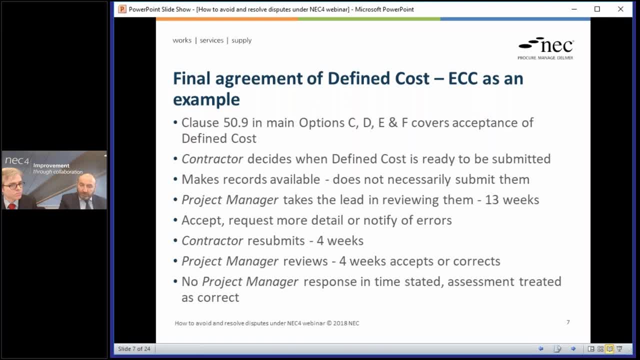 introduced is a way of agreeing defined cost on a rolling basis. so this applies in the cost reimbursable options, CDEF, where payment is made based on defined cost plus fee and the process covers under clause 50.9 how the contractor can propose that elements of defined cost are signed off, are closed out and agreed. 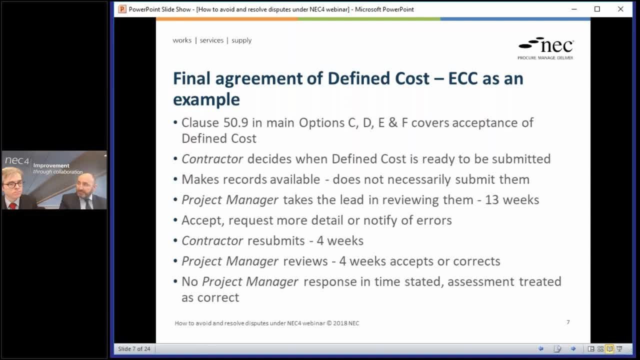 so the idea is the contractor decides when that element of defined cost is ready for submission. ultimately it's their records. they have to be comfortable that they have all the invoices in. they've settled any disputes with suppliers or subcontractors so they can definitively state what that element of defined cost is. they put that forward to the project manager. 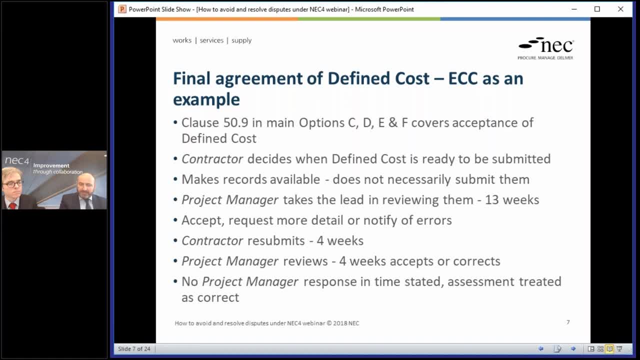 make the data available for the project manager to review. so i'm not expecting here for the contractor to submit boxes and boxes of files, rather make them available, possibly electronically, for the project manager to inspect. the body manager has a 13-week period in which to respect. 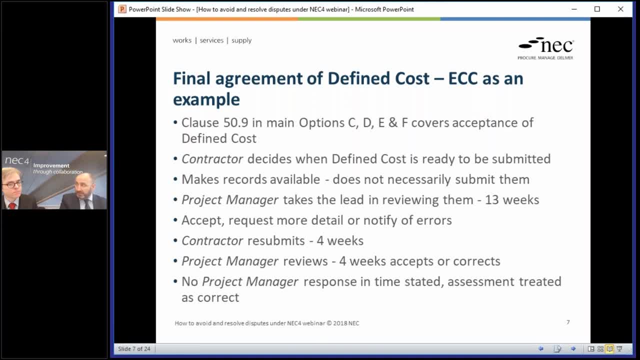 so inspect those records. that's a maximum period. they can do it quicker than great. on the back of that, the project manager either accepts it or requests for more information if there's a lack of detail in certain areas, or ask for things to be corrected if the project manager believes them to be wrong. the contractor then resubmits within four weeks. 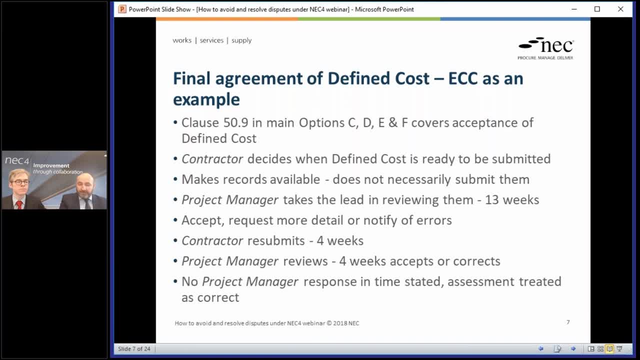 the project manager has a further four weeks once those amended, revised records are provided, and again the process is either to accept it or issue a correction to it. so the budget manager doesn't have to accept it. they can say: this bit's okay, but this bit is wrong because- and change it. 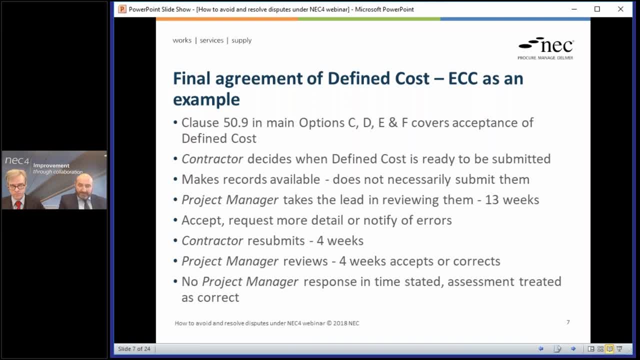 but the idea being that through this process you do have, in effect, a closed out element of defined cost not suited to being reopened and it just means that as you progress through the project you can close out defined costs for the project cost. so at the end you know, hope there's very little work to do to get the final amount of. 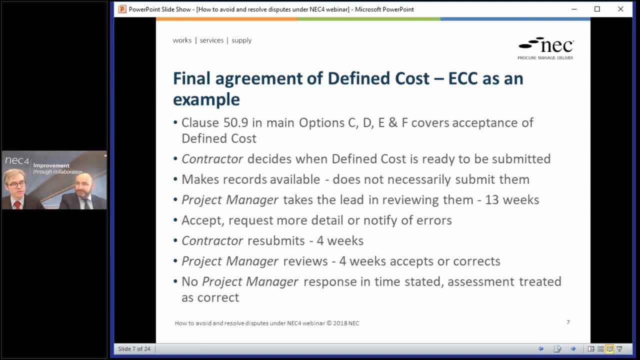 defined cost plus fee agreed. So that must take the pressure off the final assessment process. if you've already agreed on the defined cost as you go along Absolutely, and I think also it will hopefully give more security and comfort to both parties over what that defined cost is. in that 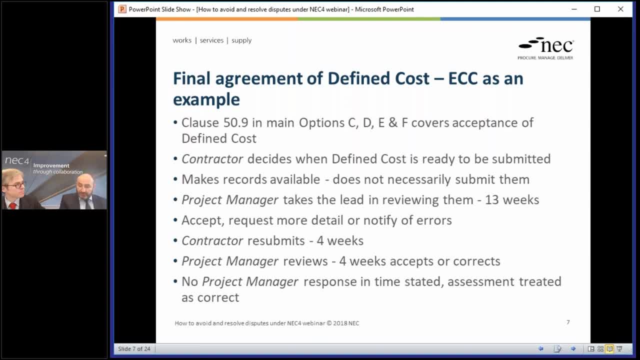 there isn't a risk that you're going to get a lot of disallowed costs if you're the contractor at the end of the project, suddenly being taken out when you didn't anticipate them, and also that when you've closed out an element of accounts for an element of work or for a period of time. 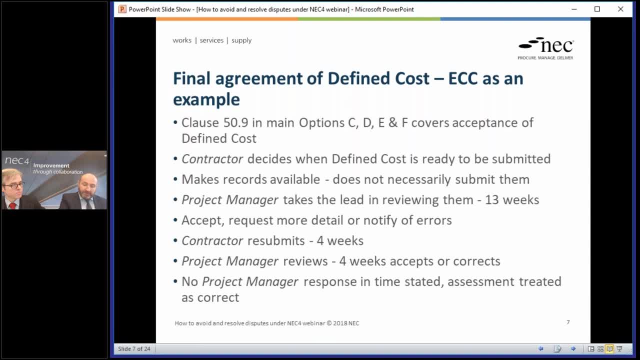 the contractor then can't come back against that. So you know, you've got to be careful about exactly how you stipulate what's being agreed and what the coverage is of those defined cost records. The idea is, once they've been closed out, they are fixed, they are final and so, as you say quite 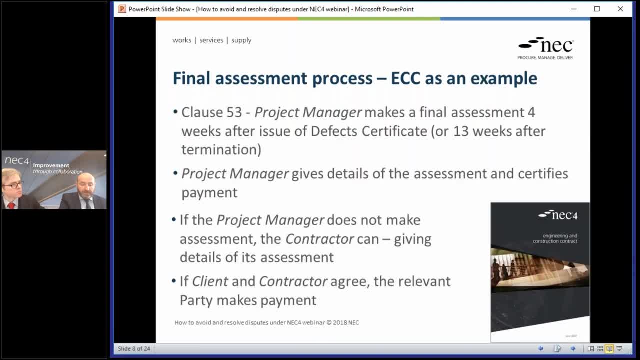 right, there's less to agree at the very end, But then you still do need a final assessment process in some way. Yeah, absolutely. I mean- I think this was an issue that did come through within any C3 feedback- that there wasn't a way within the contract to actually conclusively close out the financial. 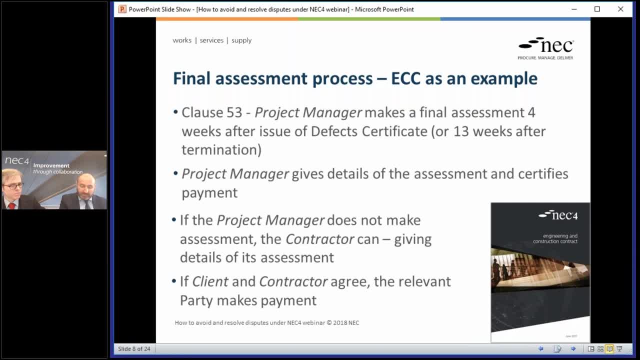 the final financial arrangements between the parties to actually close out the defined cost plus fee, so it could never be reopened to close out the total of the prices. so someone couldn't then try and claim retrospective compensation events And obviously there are provisions trying to stop that anyway, but there was still a risk around this. So in any C4 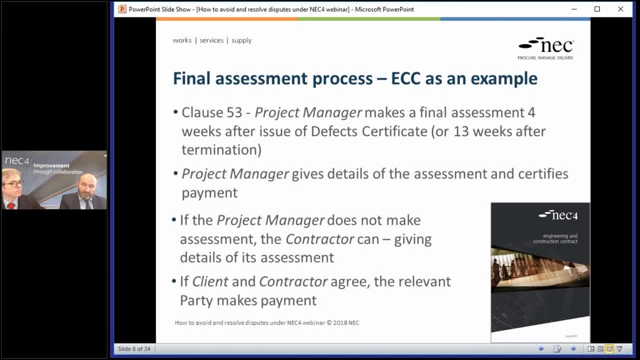 we brought in clause 53, which has a requirement for the project manager in the first instance to make a final assessment within four weeks of the issue of the defect certificate, which would normally be 12 months after the works themselves are complete or 13 weeks after termination. 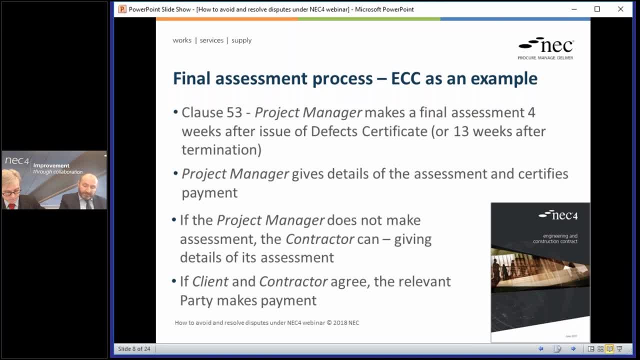 certificate if that's what's occurring on the project. So the project manager has this duty to issue this assessment. but if they don't, then the contractor can do the assessment. Whoever does it has to give details of how they've made the assessment and the if the parties agreed. 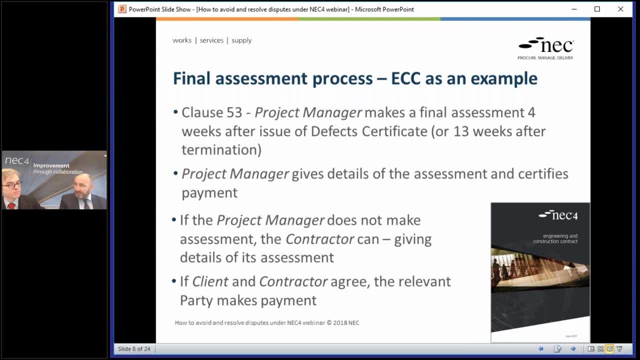 to the assessment made again by either party, the payment is made. normally that'll be from the client to the contractor, but it could be from the contractor to the client if there's delay, damages or something else. that is now making it into a negative payment. So it's quite a structured 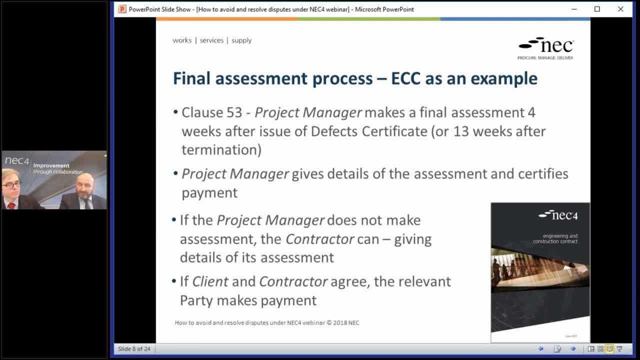 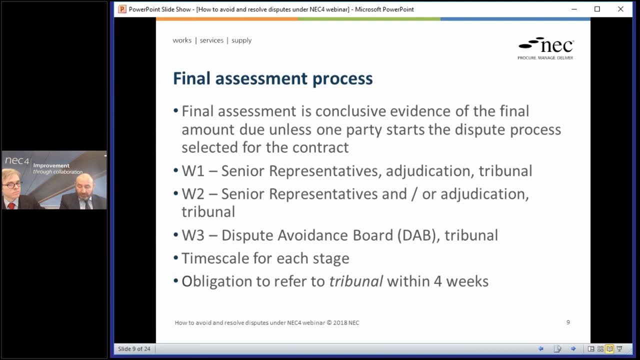 process. project manager is in the lead. if they fail to do their function, maybe they're no longer engaged by the client. they're not involved. contractor can do it. but the key thing is when either party issues that the other party has to say whether they agree or disagree with it, or rather if they don't disagree. 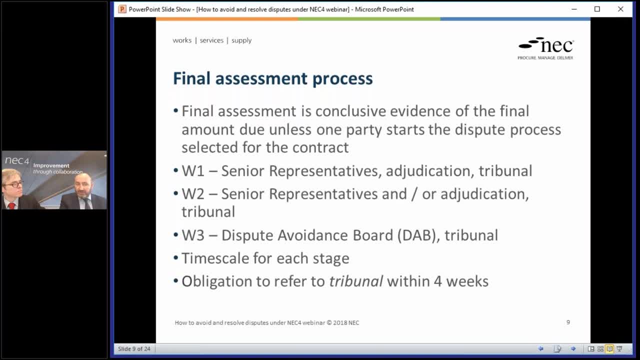 with it the final assessment is taken as conclusive evidence of the final magnitude of the contract Right. so it's the same principle as in our UK Construction Act where, on a monthly payment notice basis, if the contractor issues his payment application and the PM doesn't apply. 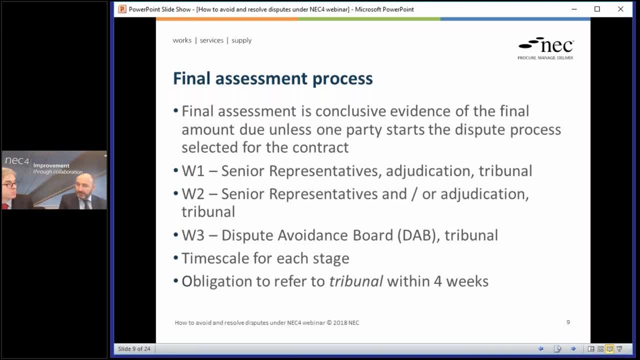 then that contractor's payment application is taken as the payment for that month. So it's effectively applying that, but in the final assessment context. Yeah, so the idea is it's quite a simplistic process, but it is creating this mechanism of forcing the parties to either formally disagree or either formally agree with this. 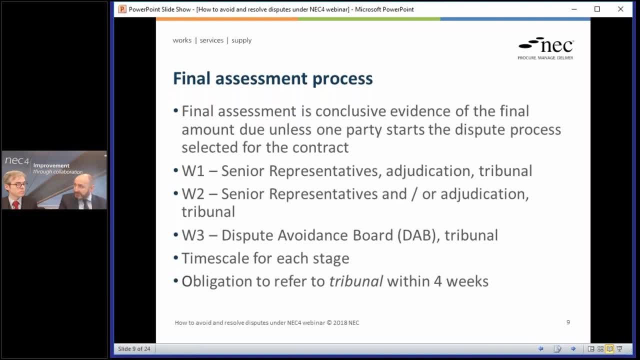 if they're silent, That's then going to be agreement. After the end of the timescales in the contract- I think someone's just raised a question there around- does the contractor have to remind the project manager they failed to issue the final assessments? 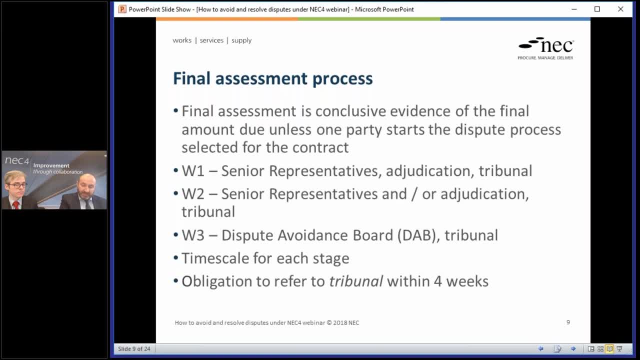 And the answer is no. the process is: project manager has a duty to issue it. if they don't, the contractor can issue it Back to 10.2. then mutual trust cooperation: there's nothing stopping the contractor saying it's been four weeks, so we'll come up to the four week stage. have you done it? project? 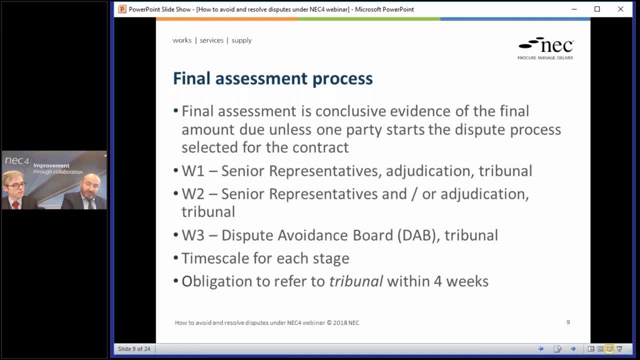 manager And there's nothing stopping again looking to work together. So we've got to work together to do that. but if the PM doesn't do it, the contractor can issue it. But whoever issues it, the other party can raise an objection to it. but they have to. 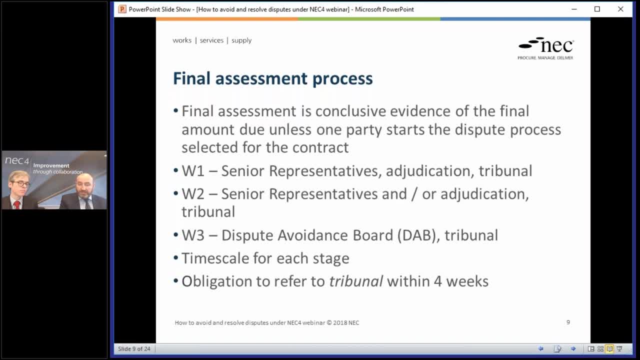 raise that formally and they have to then start one of the dispute resolution processes under the contract Right. so it's not just a pay less notice or pay more notice, depending on which side you're on. it's a formal dispute at that point. 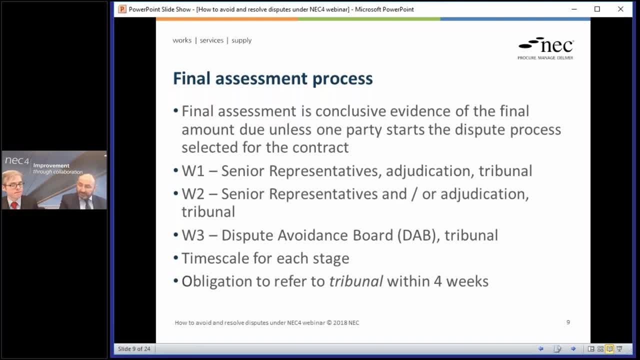 Yeah, the idea being that we don't want things to drift and people either be to be silent or agree to disagree. It's, you know, almost railroading the parties into. if you don't agree, you have to formally disagree, launch a dispute resolution process, and that way we are now into a mechanism with 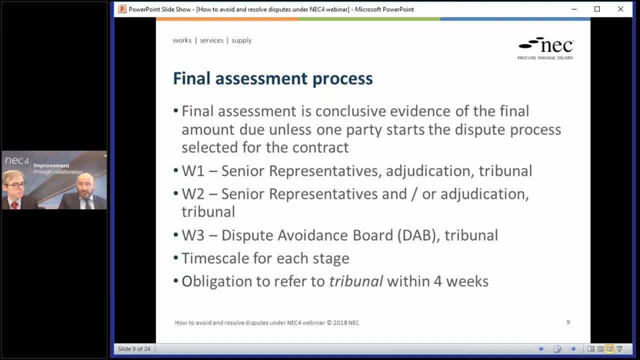 set timescales to get to a final conclusion, Because the way it works is you do each stage of the dispute process and you have to move into the next one within a set timescale. So, for example, in W1, the senior representatives will meet and try and decide the issue. 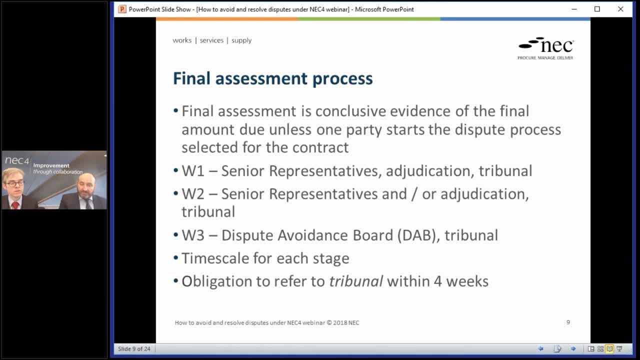 If they fail to achieve a decision on that, you would have to launch the matter or take the matter to adjudication if you disagreed with anything they agreed or did not agree to At the end of the adjudication. if a party is unhappy with what the adjudicators decided, 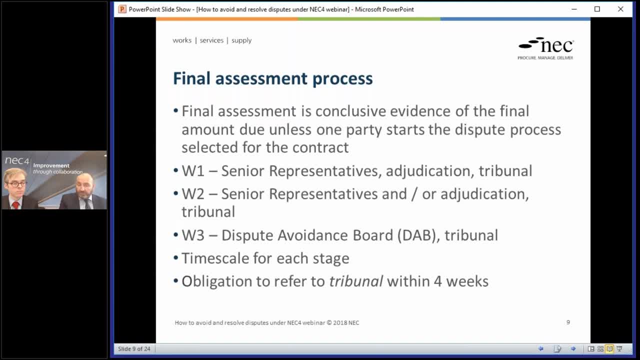 again. they would then have to launch an action with the tribunal within a four-week period, And that four-week period might look narrow, but I think overall it isn't. I mean, it's not as if within that four weeks one has to present all of one's evidence and 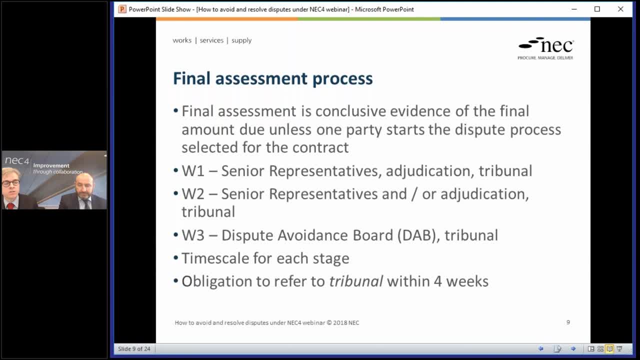 one's case and one's delay analysis and one's technical analysis. Yeah, And people are going to be very confused. Yeah, They're going to be very confused. You have to put a claim form before the court and that's a two-page document. 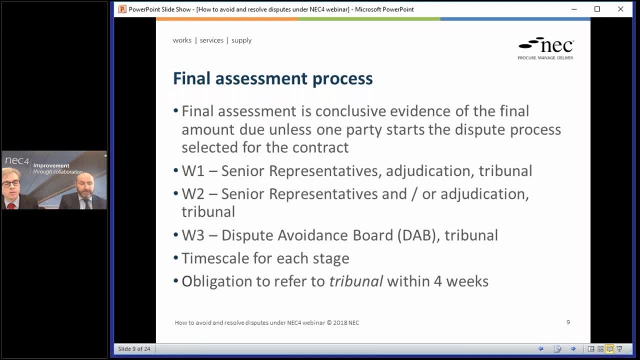 I mean to refer to a tribunal. we'll get onto the different types of tribunal later on, But, simplistically, either you have to put a claim form before the court, and that's a two-page document, or you have to commence an arbitration, and that can be a very simple. 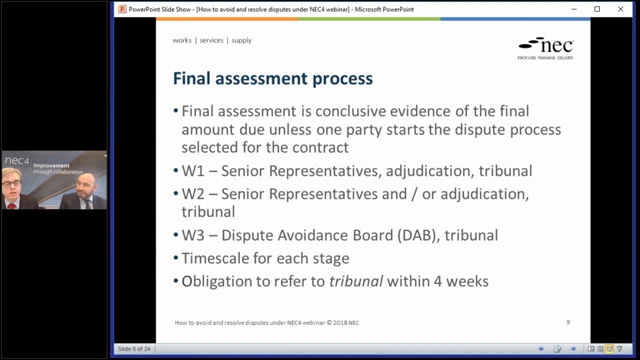 document. So the four weeks has no particular magic to it, as I understand, but it is going to be long enough to raise a formal dispute. Yeah, And obviously your two parties to a contract can agree to various things. Yeah, Yeah. 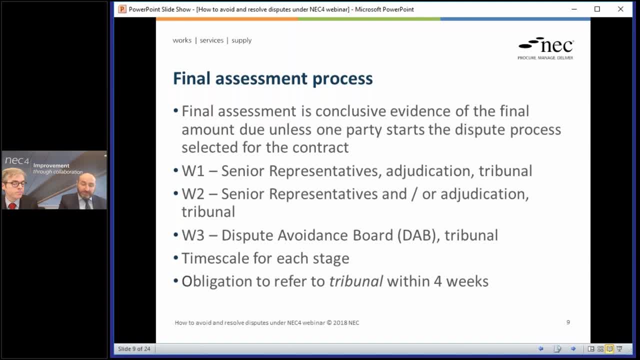 So they could always agree to extend that period, Perhaps if there was going to be some further negotiations. perhaps the adjudicator has decided some substantive issues. there's a few minor issues left. Well, actually, maybe they could agree to hold on going to the tribunal, mutually agree. 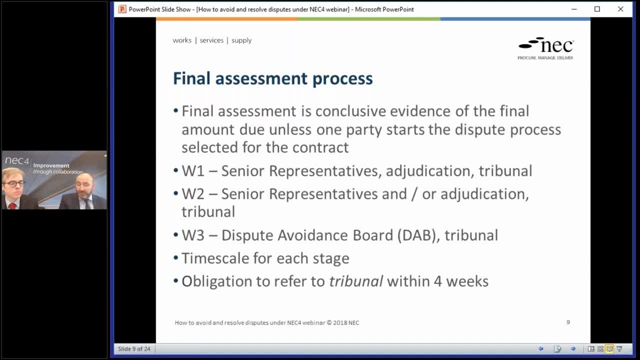 to have an extended period to try and settle those outstanding issues before launching into that process. That's right. This is really to deal with where one party is not engaging, is not providing a response, and the other party can force it through to a conclusion. 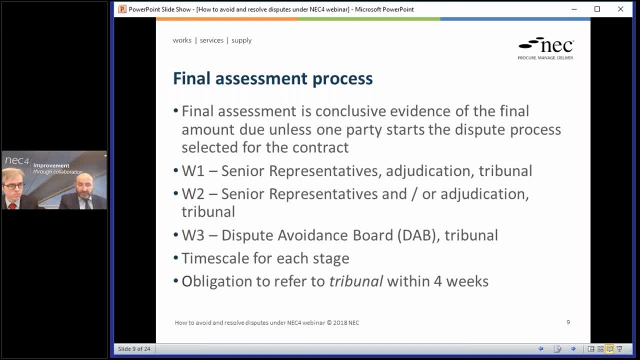 Yeah, Which is similar to the vast majority of the procedures in the standard contract: the ability of a party to drive things to a conclusion if the other party does not engage. We see in compensation events program acceptance. now A couple of other questions have come in from people on the webinar. 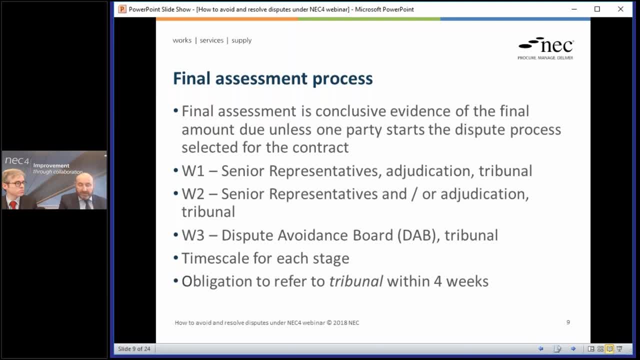 This process in terms of the final assessment, clause 53,. that applies to all of the main options and we have similar versions of this in all of the contracts. So all contracts in the NEC- We have all the main contracts- have this final assessment process and it covers across. 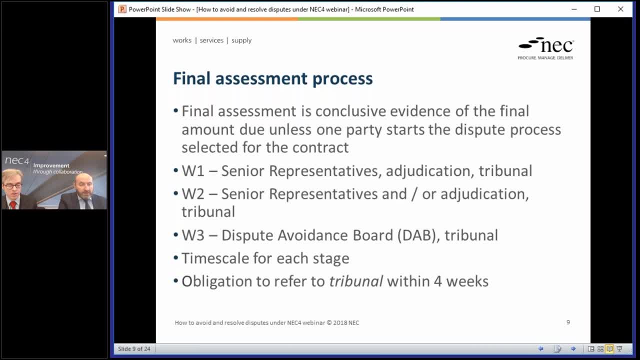 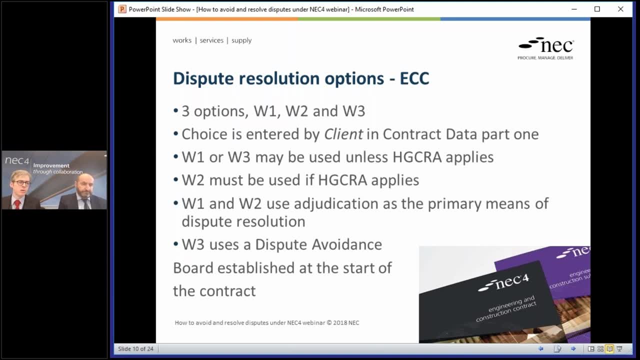 all the main options. Okay, I think probably good now to work on to the dispute resolution options, because we've got W1, W2, and W3, and effectively those are a sort of NEC code for different- they're not different- types of dispute resolutions in themselves, they're different mixes of. 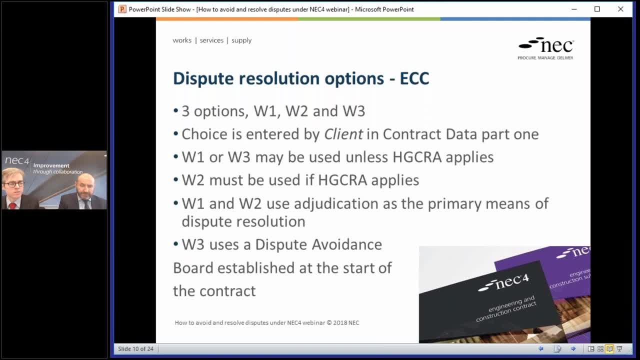 dispute resolution styles. We'll explain that. The first thing to think about is what is going to be my choice of option As a matter of principle. it's entered by the client, First part of the contract. data is provided by the client, the employer, and it's that. 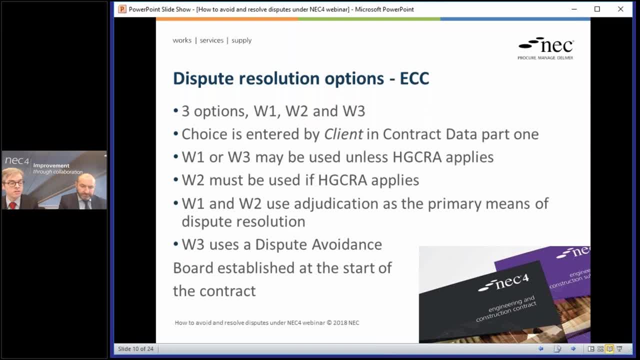 choice. I mean, of course it can be negotiated if the contractor has any sort of leverage in that respect. Frequently clients, if they're doing large projects, like to have a single option with all of the contractors so they know what they're doing. 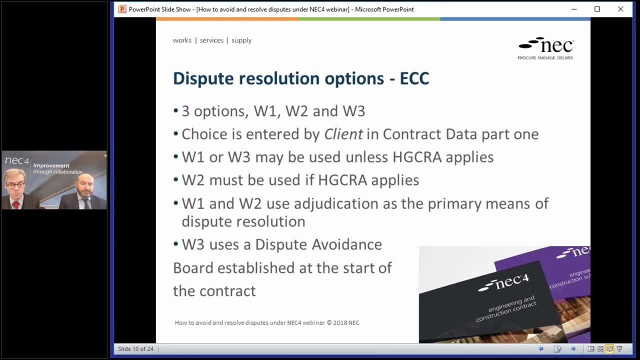 So it's frequently just imposed- for want of a better word- by the client in contract data. part one. Now, the reason why there are several choices is simple: that different projects have different requirements, but also one has to have regard to the prevailing legislation. 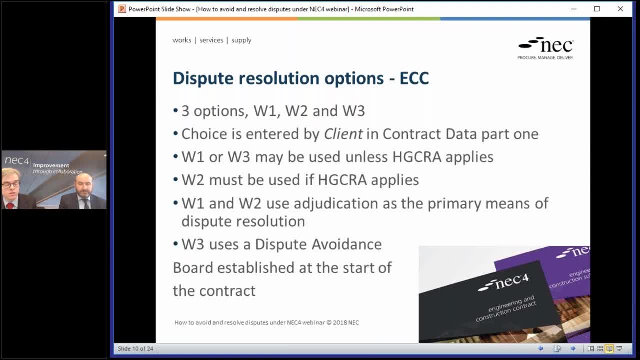 Here in the UK we have the Housing Grants Construction Regeneration Act that we typically just call the Construction Act, And that requires It requires for all construction operations contracts in the UK that adjudication must be available, And so a specific provision has to be made for those, and that's the W2 has to be used. 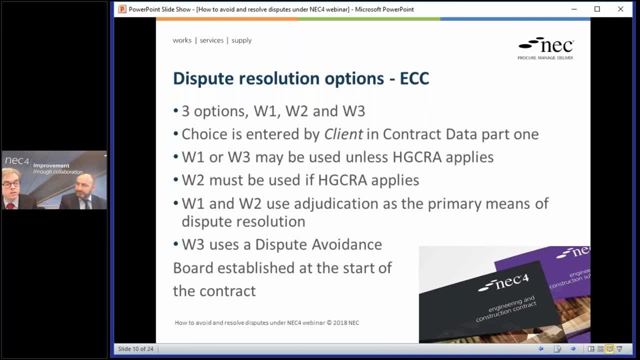 if you're construction operations in the UK, because adjudication is available in W2.. The others- W1 and W3, can be used if you're either in the UK but not doing construction operations, or if you're around the world and you're not bound by the construction. 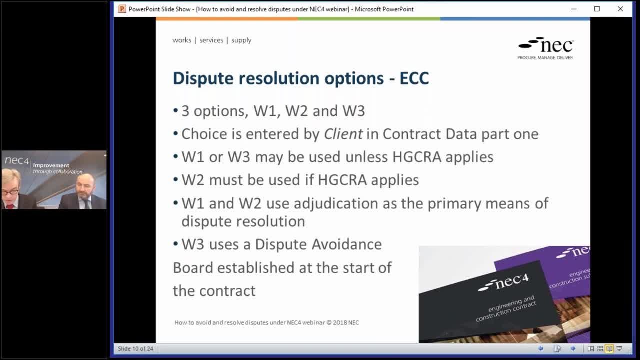 Act To simplify and we'll go through them in more detail: W1 and W2, the main way of resolving the dispute is adjudication, and W3, there's a relatively new option. there is to use a dispute avoidance board. 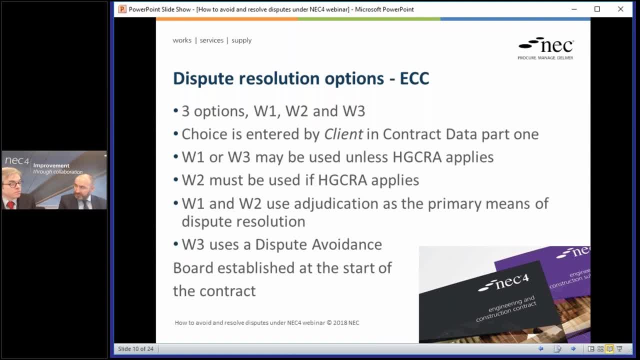 So just to recap on that, Marcus, we have a choice of three options in the ECC. I think it's worth pointing out that W3 only appears in the ECC contract. It's not in the PSC, the TSC, the supply contract. 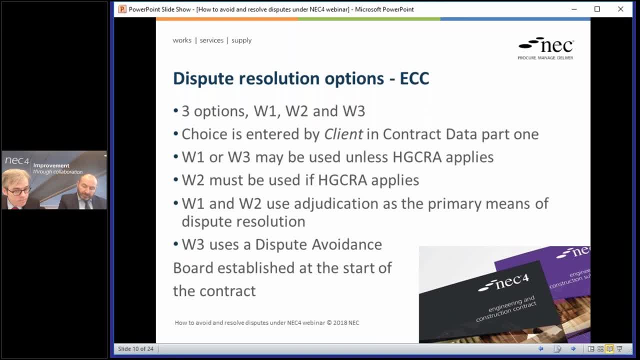 So it's not in the PSC the TSC the supply contract. It's not in the PSC the TSC the supply contract. So it's not in the PSC the TSC the supply contract. So it's not in the PSC the TSC the supply contract. 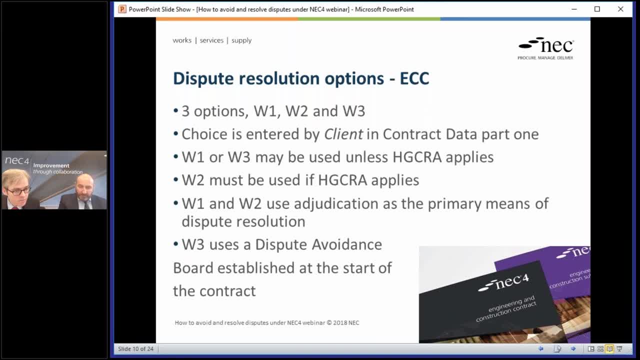 So it's not in the PSC, the TSC, the supply contract, And so we have these three options, As you already outlined. in the UK, if the work you're doing is covered by the Housing Grants, Construction and Regeneration Act, you don't have a choice really. 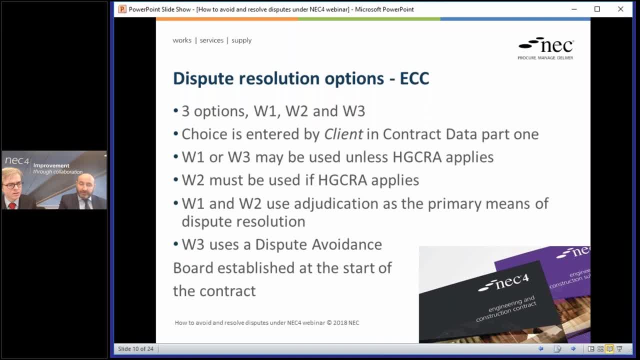 You have to pick W2 because that is the only option of the three that is compliant with that piece of legislation. If you're operating outside of the UK or undertaking work in the UK not covered by the Act, you have a choice of W1 or W3.. 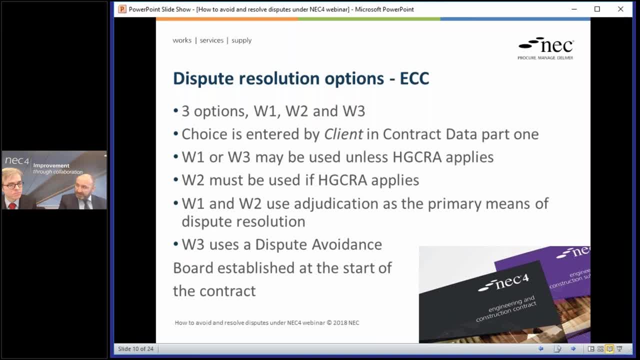 You could still use W2.. But actually W1 and W2 are very similar And the reason why we have W2 is actually to meet the requirements of the Act. And if you were working outside of the Act's jurisdiction, the board of the NEC would recommend. 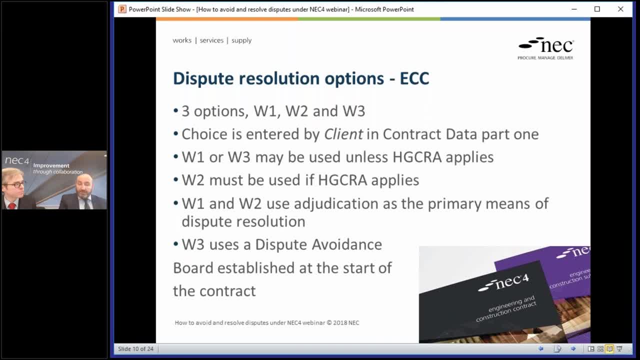 selecting W1.. The feeling is that's a better process. It has a reference table for taking matters to dispute. It has slightly simplified processes, So the view being that that is a better adjudication process than W2, but we need to have W2 to comply with the Act. 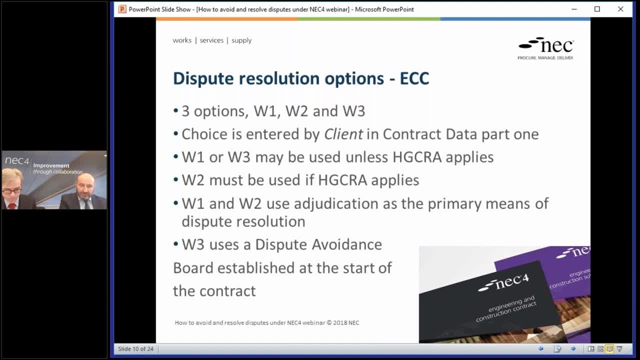 So overseas, outside of the Act's provisions W1 or W3.. If you want adjudication, W1, W3, we'll talk about in a bit more detail shortly. So, Mark, back to W1 and W2.. Yes, back to W1.. 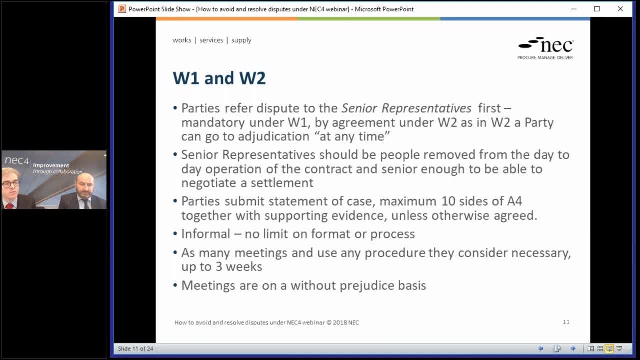 And there's been a question that's come in about the senior representatives element. I mean this mode of dispute resolution will be familiar to those using sort of tiers. Yes, I mean we've had arbitration clauses and the like that are increasingly common. 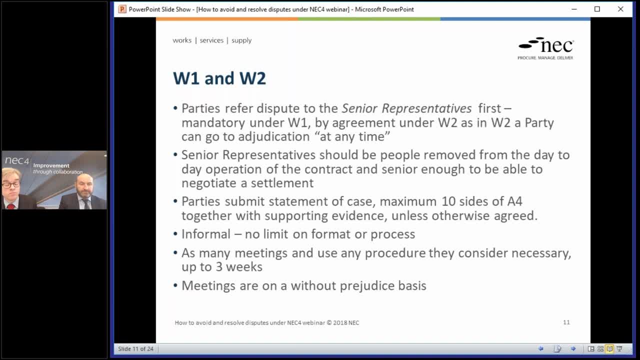 The first stage of a dispute resolution is to refer it to the senior representatives. Now, under W1, it's mandatory And, as Ian was saying, that's the preferred option, Or under W2, it's by agreement. Senior representatives to answer the question. I mean they need to be people who are senior. 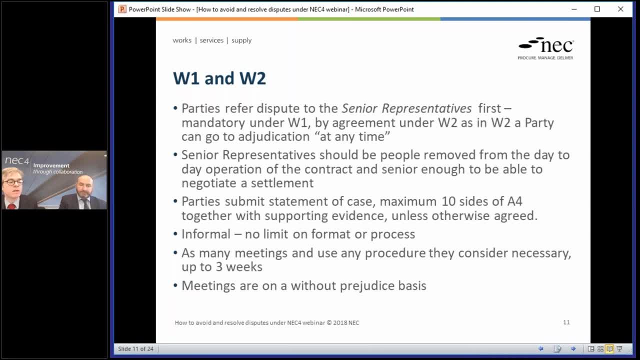 in the sense that they are removed from sight. They are removed from the day-to-day operation of the contract. Yes, They are removed from the works, but also from the commercial negotiations. The idea is that you have someone who's sufficiently senior and sufficiently separate to take a 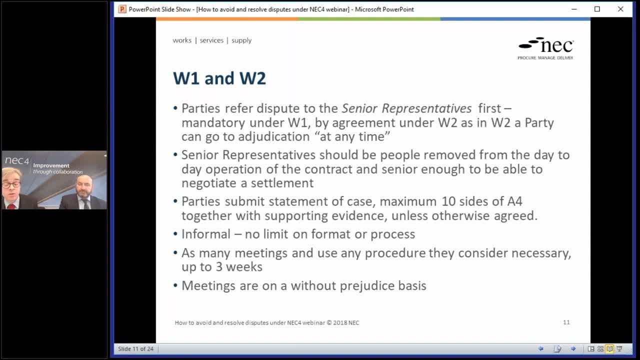 cooler view, who is not affected by discussions that may have been going on for months. people taking particular opinions entrenched views. people are possibly invested in them. We need somebody, not necessarily at board level, but at a senior level, who can take 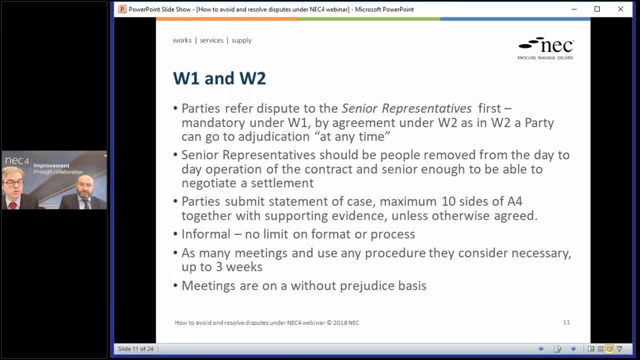 a step back and see what is the dispute worth Financially, what is it worth in terms of the progress of the project and what's most important here. And hopefully, if you get one from each side, that's got that perspective. it doesn't have. 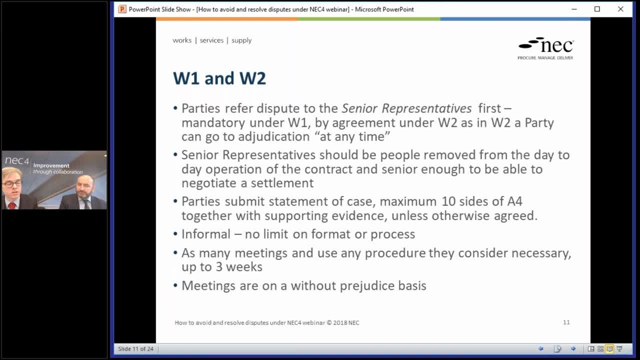 to be someone technically qualified. It just has to have somebody with the gravitas, with the seniority that can make a decision, can bring his side with him and can make a decision effectively. If you were, a good analogy is if you were going to mediation and you wanted to send. 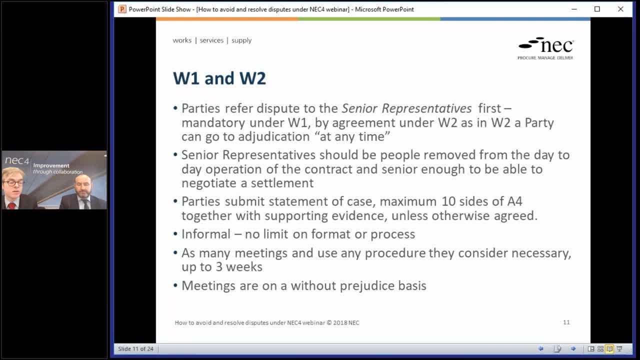 somebody along to make the decision, Ask whether to mediate- Yes To mediate- or to settle at a particular level. it would be that sort of figure. The process that's put in place here reflects the sort of people that the drafters had in. 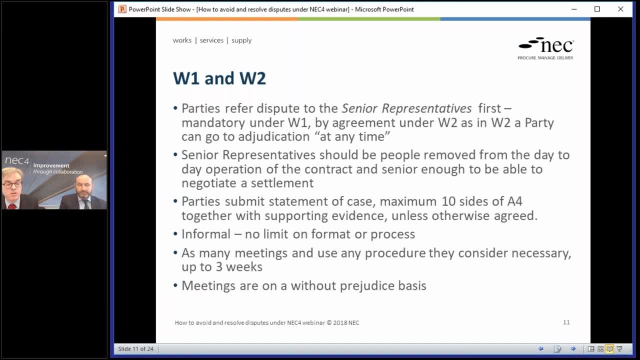 mind. It's a very short statement of case: 10 pages executive length with some supporting evidence. Parties can always agree longer, but typically these things work best if it's done on a limited amount of paper. It's an informal process. 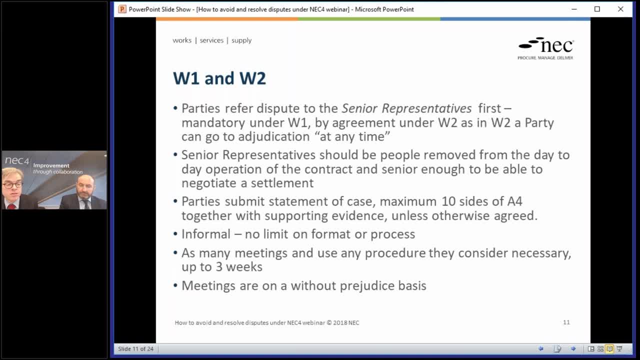 The parties can agree how it works. The senior representatives can ask for an expert to assist them. They can ask for a mediation to help work through issues. There's no limits really to it, but there is a time limit to it because of the dynamic. 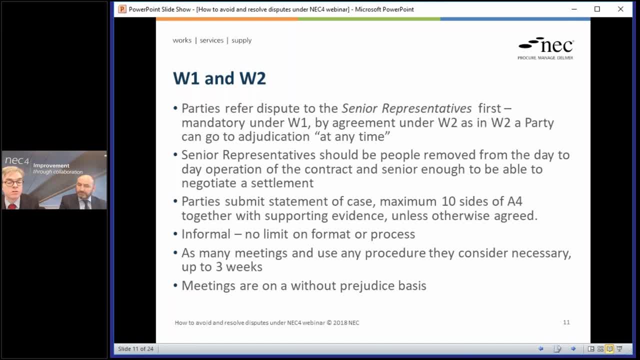 of trying to bring people to a resolution, to oblige them to act to resolve their disputes. Yes, I think it's a key thing. There is a time limit. We don't want to turn it into a talking shop where people spend weeks, months, extended. 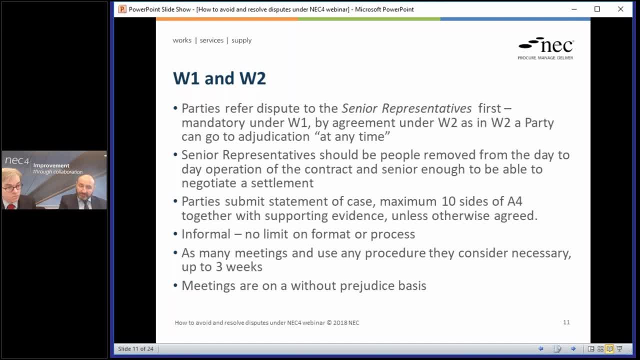 periods of time talking but not getting it Again. that can be extended by mutual agreements, but it can't be used as a delaying tactic by one side. In terms of the process, as you said, it can be very informal. We've deliberately not, within the contract, specified how it should work, because this 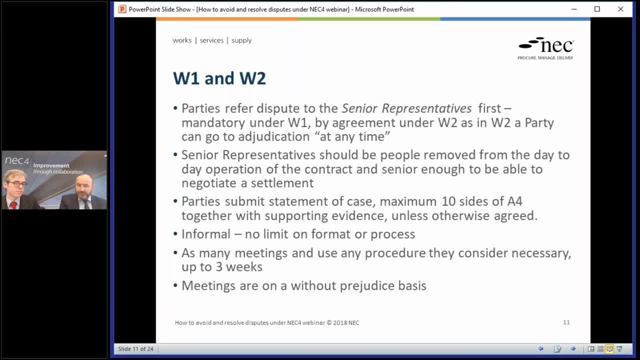 was really going to be a consensual dispute resolution process whereby the parties are looking to do a commercial deal. in effect, They're looking to agree. Can they come to a compromise, Or can they both agree A particular interpretation? I think there's a fair chance that at the end of the day, the process is very difficult. 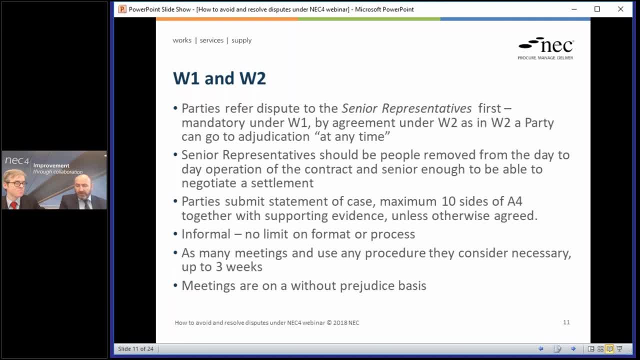 I think if you can come to a compromise, the compensation that has been made. you've got to get to that level where the parties are equally involved in the dispute. It's a very clear-cut, clear-cut, clear way of coming up with something that is in the 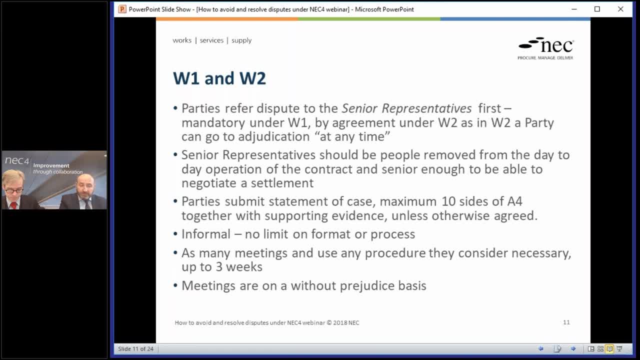 way of taking on the dispute. It's a very clear-cut approach. I think people are happy to come to a compromise, and it's a very clear-cut approach. People are happy to come to a compromise on the dispute, but I think then there's going. 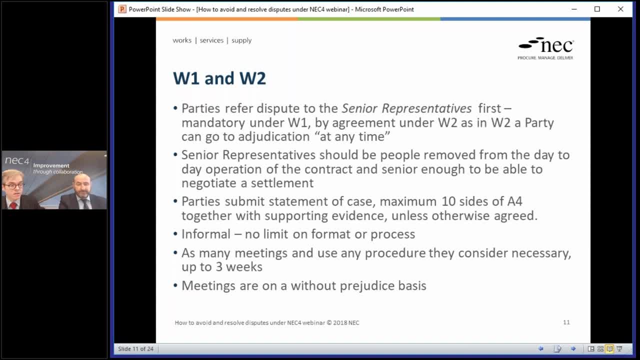 to be some kind of some sort of negotiation to resolve the dispute. If it's got to this stage, it's probably going to be an issue that isn't clear-cut. Therefore, there may be some way of compromising or coming up with some sort of deal that. 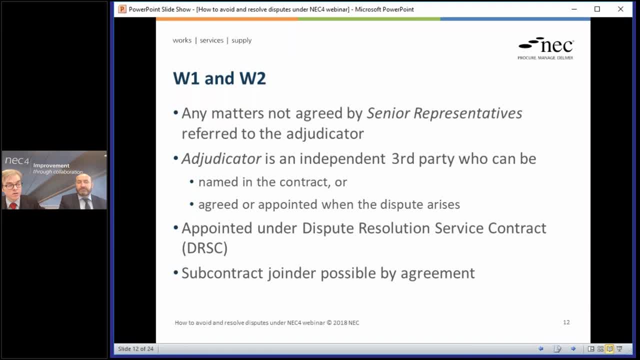 will satisfy both parties and W2. envisage that you go off to an adjudicator. Now, an adjudicator is an independent third party, completely independent of the parties. There are a few options in relation to identifying an adjudicator and we would recommend. 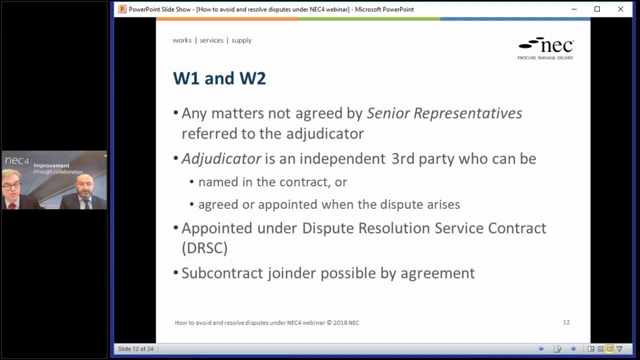 everyone give very careful thought to this. The first is to name them in the contract: either an individual, or sometimes it's useful to mention a panel of people who can potentially be adjudicators to deal with availability issues and so on. That can have drawbacks as to availability, etc. or 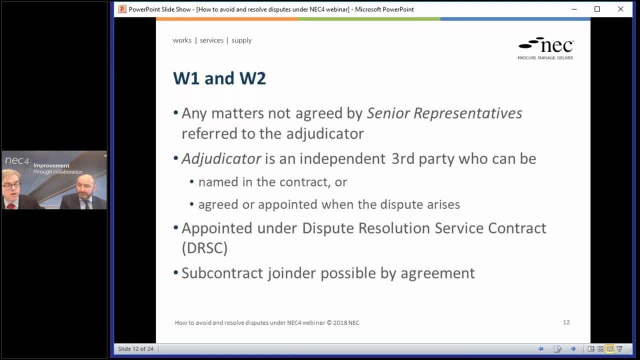 indeed, it may be impossible to agree at the outset of the contract. A very widespread method as an alternative is to agree an appointing authority, be it the ICE or the RICS, several appointing authorities that will have a panel of qualified individuals with the requisition. 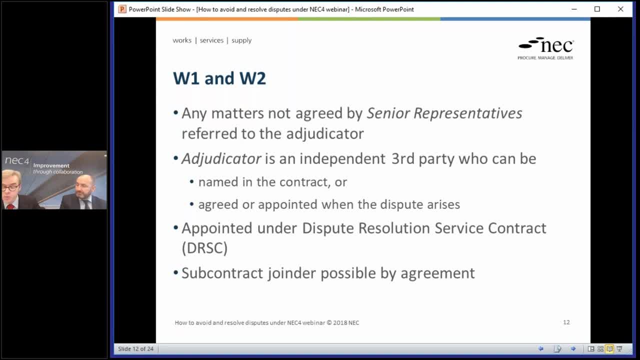 its skills. Under the NEC Suite, it's now possible to appoint an adjudicator under a dispute resolution service contract. We'll get on to that, but it's appointment terms, as that deals with the terms of appointment, and it is possible to join in your subcontract disputes as well, simply by a. 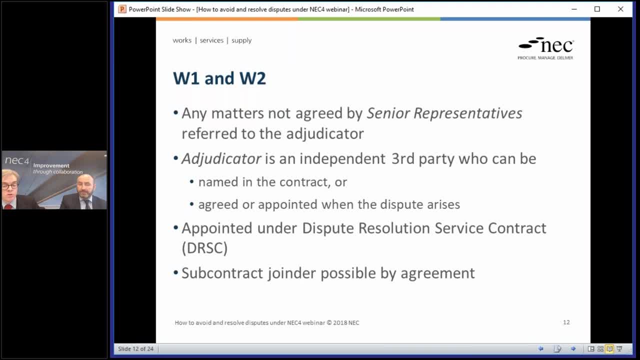 matter of agreement, So that that's not something that should be done lightly, because it creates a risk of being a subcontractor. So that's a really important aspect for us and we'll get to that As well. it is possible to join your subcontract disputes as well, simply by a matter of agreement. So that's not something that should be done lightly, because it creates a compromise between the parties. 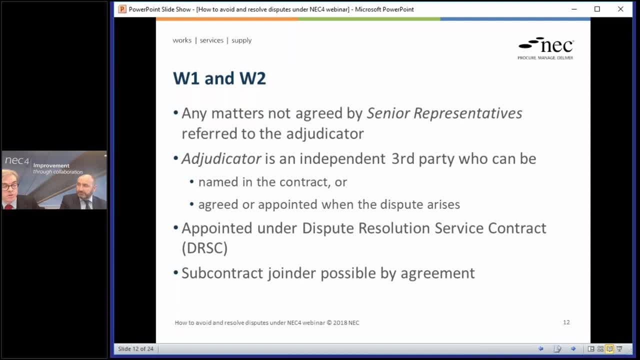 creates a much more complex dispute which might not be suitable for adjudication, but it's something that's possible by agreement, okay, so yeah, come back to that idea. in terms of who should be an adjudicator, i think you know there's no specific requirements in the contractors as to any 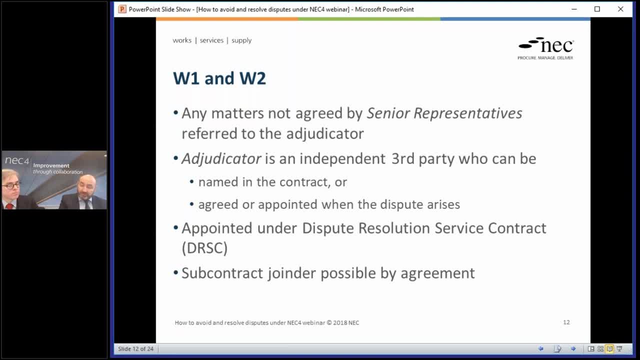 particular skill set of that person. the contract simply allows the clients in contract data, part one, to name an adjudicator, so that could be someone who obviously they believe has the skills to act in that capacity. you mentioned that. you know you also have to include as well as if you 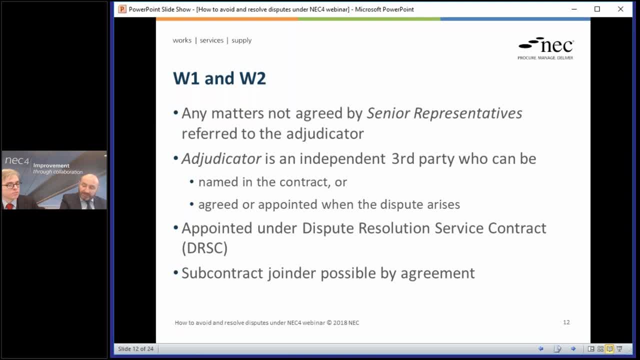 name someone, or even if you so, if you don't, even if you do name somebody in the contract data, you still have to put in a nominating body, because there's a chance, if you do name somebody, that they may not be available when the dispute arises. there's very tight time scales for adjudications. 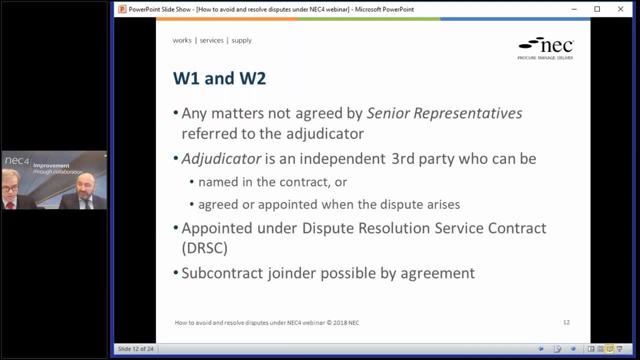 in which they take place. if that person can't act immediately, you would need to find an alternative. hence the need to include a nominating body. and they say some people do actually leave it blank and have just a nominating body because, again, there may be a perception- if the client 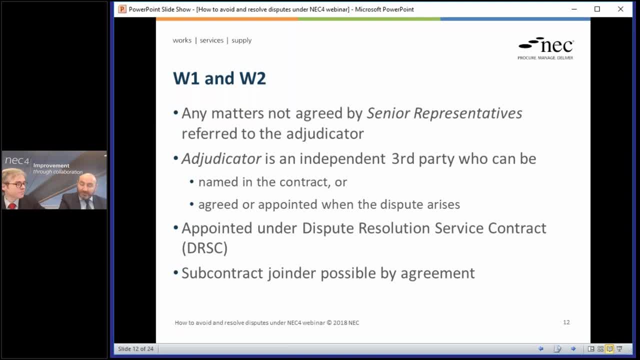 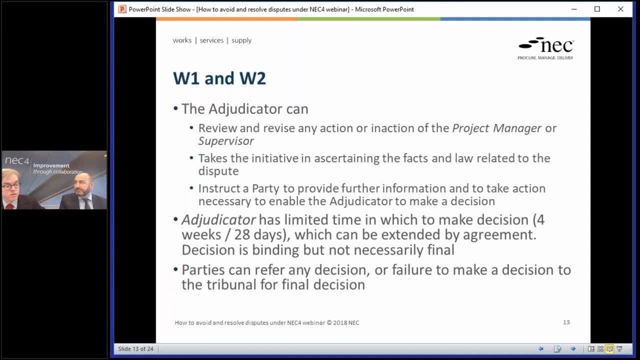 names a person, will they be truly an independent third party or do they have some existing relationship with the client? that's right. a nominating body can, in the right kind of case, look at the notice of adjudication, see what sort of dispute is and find someone that's got suitable. 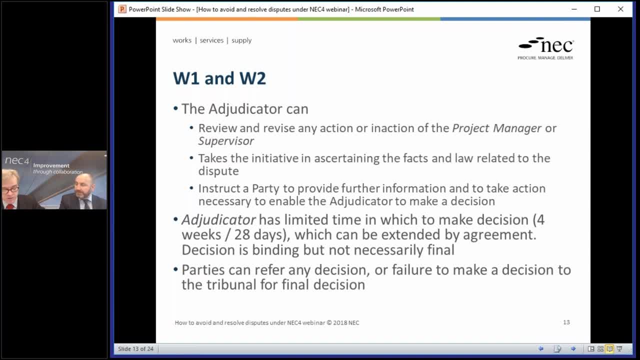 suitable skills for that, so that that gives a wider range of possibilities. yeah, and i guess the only downside to that course is the parties are then putting their trust in that nominating body finding a suitable person, whereas if they can both agree mutually to somebody, that's going to be even better because they'll have somebody who 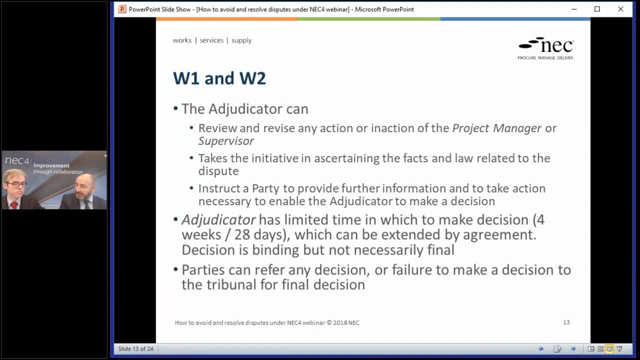 they are both happy with and they both believe has the ability to act as the adjudicator. now. now just about the powers of the adjudicator. they're very broad. um, the adjudicator can review or revise any action or inaction of the pm or the supervisor. uh, and can can hear the dispute. uh, find the facts. 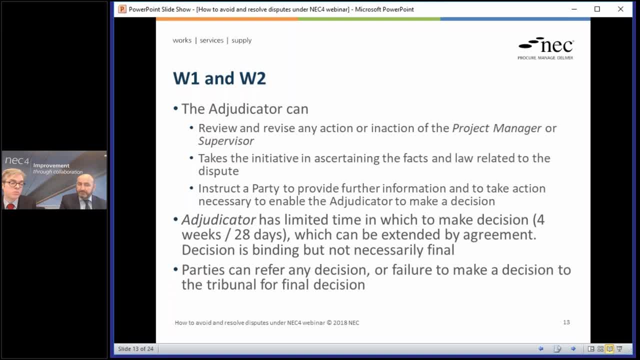 uh hear the law, uh really, in any way he or she considers appropriate. uh. document production, or disclosure as we call it here, uh is not very normal in adjudication processes. however, an adjudicator can instruct a party to provide further information. it's um. it's a classic inquisitorial process where the adjudicator has a range of powers to ask for. 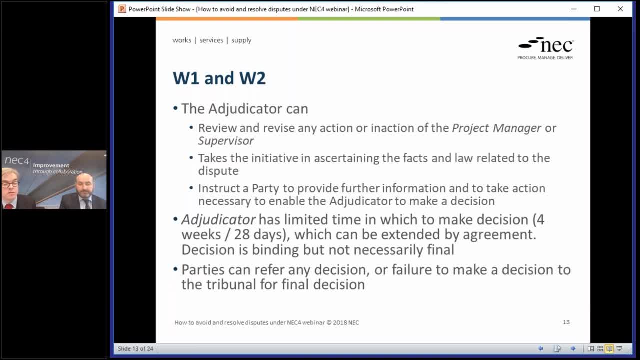 anything he or she would require um and the parties have agreed to to cooperate with it and should do so. um. one of the more difficult aspects of adjudication procedure is the time scales. um, as a matter of the the act here, um, there's limited time to make the decision, and 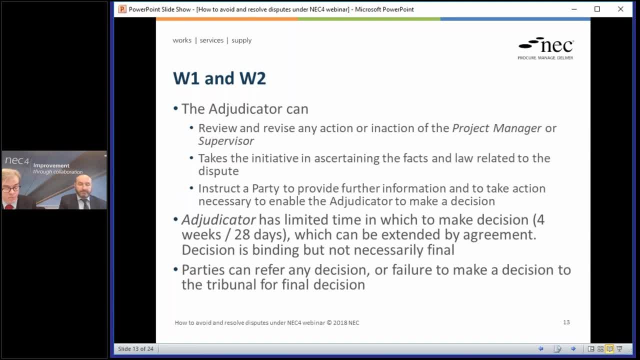 we've sought to make it a situation where the law allows the justices, the actors, to work alone, uh, in order to get the necessary minutes to correct the crimes that they should have committed. but there are certain cases where the case can be Проститутive. in that case, either, it's a process. 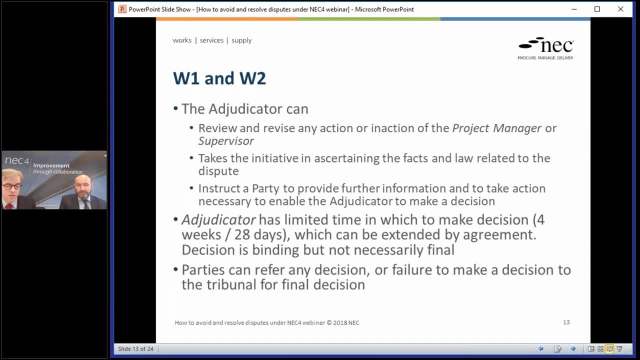 or it's a case where um we have to do it and then have toаются a procedure um which is bottle of water. the case is usually a 28 day trial. that typically 28 days from the referral. um now that entirely within 28 days, you can think, for example, complex extension of time claims or 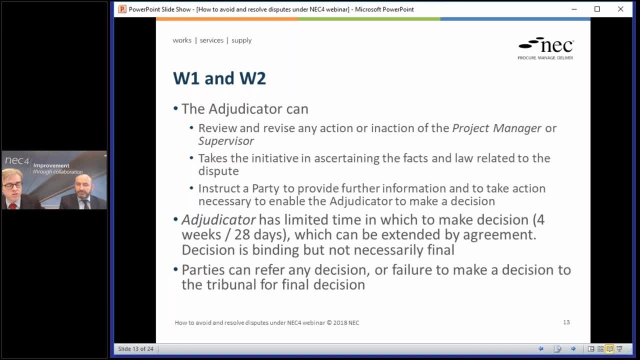 defects claims or, you know, a large package of variations. these sorts of claims are very difficult to do in 28 days. So could the adjudicator say I can't deal with this, therefore I don't have to give a decision, or do they have to give a decision? is that the nature? 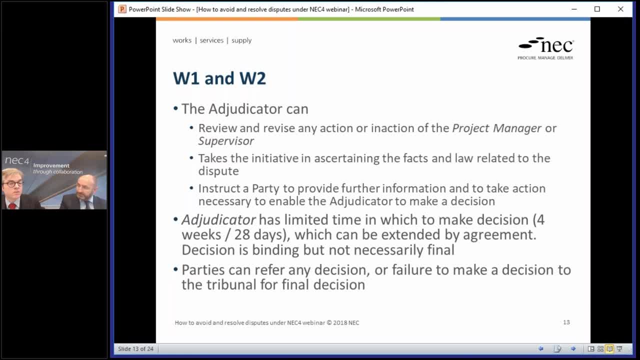 of the process. No, it's actually open to the adjudicator to say: I cannot deal with this within 28 days and therefore I'm accusing myself and I won't hear it. Well then it'd be a case having to put another adjudicator through that process again. so ultimately, even with a complex 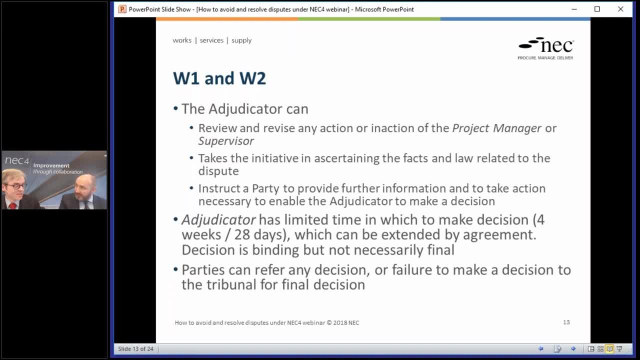 or large dispute, you'd have to go through and get to an end of that process. You would, and eventually you would find an adjudicator willing to take it on. Okay, and I guess the issue that then coming back to say they have a limited time scale, is there an issue about rough justice here. 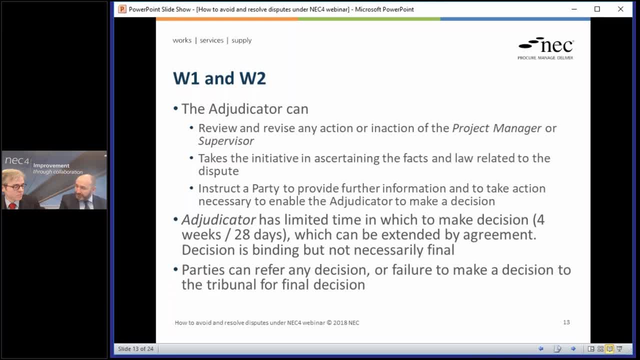 could you know, a decision be rushed or forced? that maybe doesn't cover all the facts or all the debates and arguments that could be put forward? And it does happen, And we shouldn't be too embarrassed about admitting that it does happen. It was always. 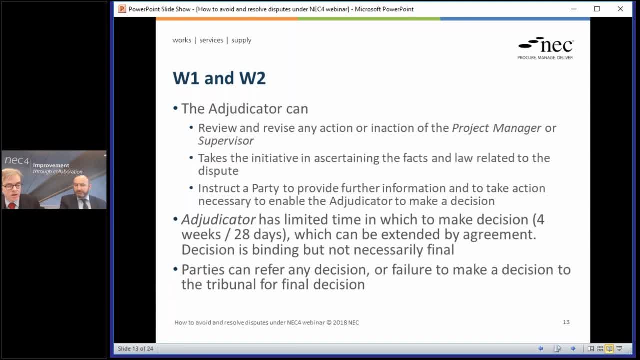 expected that that would happen with these more complex cases. Adjudicators are forced in those cases to take shortcuts to you know. to take a variations example, to take a sample, I'm just going to look at the top 10 and, on the basis of my decision, of those, I'm going to apply that. 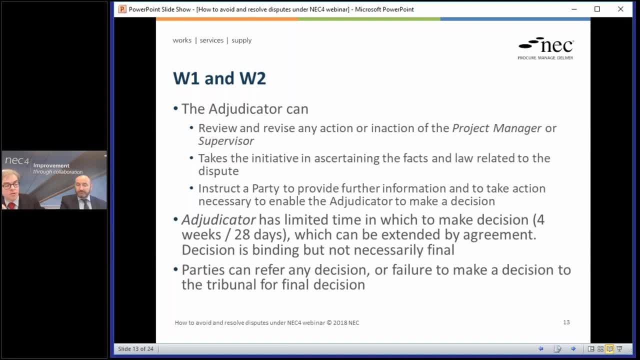 pro rata through the rest. That's extremely rough justice to take extension of time decisions purely on the basis of the programs with a very little investigation of what actually happened. That's the way it is. But I mean, you know the core of what happens with an adjudication decision. 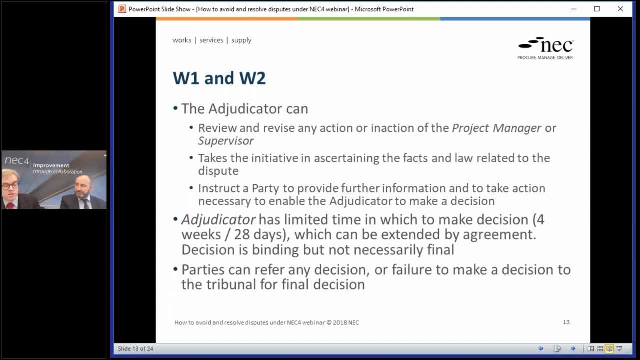 is. it's binding but it's not final. The ultimate saving for the procedure for these over complex cases is that if one party isn't happy with the decision, it can be referred up to the tribunal for a decision which would be final. Okay, so decision is binding, but not final. When you say it's binding, 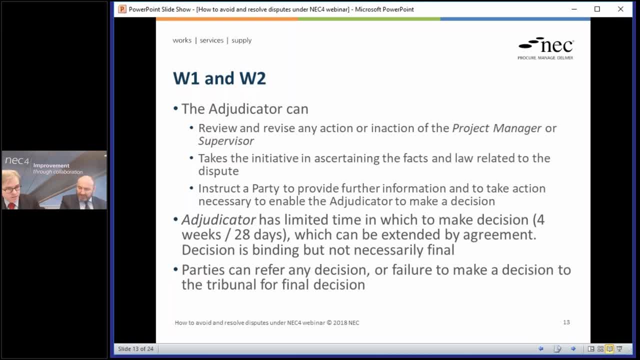 and it's binding as a contractual obligation. so similar I guess to possibly in the course of the dispute, which was someone disagreeing with a contractually binding decision that they disagree with, such as a project management assessment of a compensation event. So how would somebody enforce or get a party to comply with the decision of an adjudicator? Well, that's right on a very 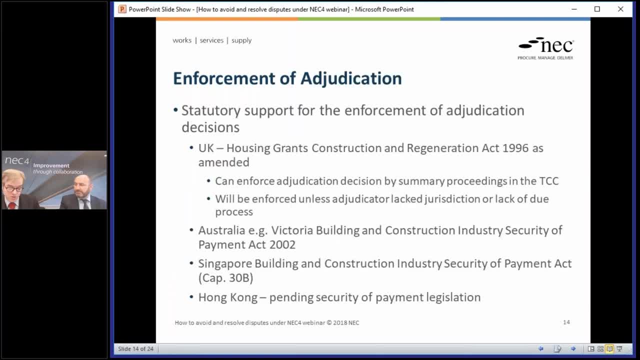 basic level. you start with a contractual claim and then, once you've got an adjudication decision, you have a contractual claim. So you're right in saying that. you know, conceptually it doesn't advance the party much. Now what you know, the law has recognized this and how we take that. 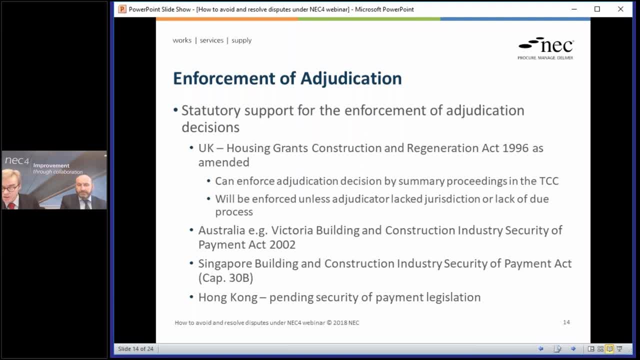 forward is that the statutory support for the rapid and no questions asked enforcement of adjudication decisions. Now this starts in the UK with our act- the full title is now up there- which makes provision for summary enforcement of adjudication decisions in technology and construction courts here in the UK. That's a fast-track procedure- can be done within a month. 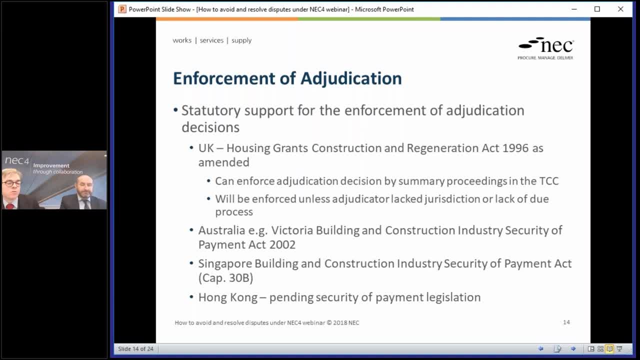 and, crucially, the courts won't go back to the merits of the decision. They will take the decision, say this is a decision, this point has been decided by the adjudicator and we'll enforce it, unless there's a lack of jurisdiction, whether he's gone ultra. 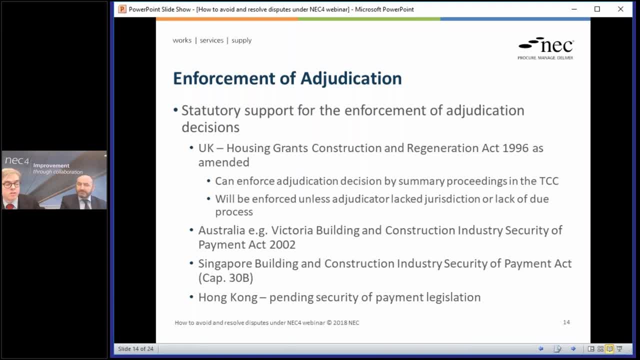 virus beyond his powers or there's been a lack of due process or bias or something serious of that nature. That's the model In Australia also. that's on a state-by-state basis in Australia, where they have similar legislation to enforce adjudication decisions. We've cited Singapore as 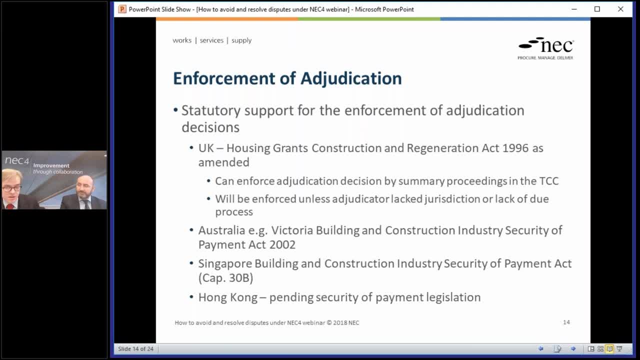 well, Hong Kong it isn't there yet. There's a process in place to enact that legislation. It has taken some time, as the local legislature decides between the different models of legislation, but we're hoping that soon there will be legislation in place so that in Hong Kong you can get a fast 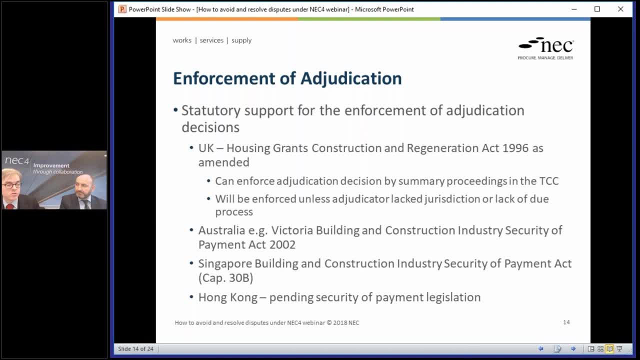 track enforcement in the courts and therefore convert your adjudication decision into a court judgment very quickly. Okay, so I guess what I'm saying is that in these particular locations, statutory support enables a party who is successful in adjudication to get that decision complied with very quickly with that court support. In other locations where you don't have, 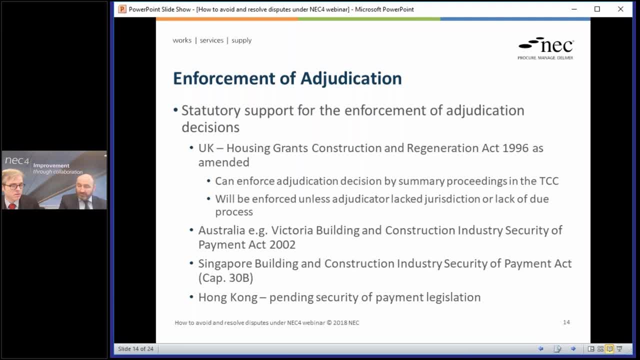 that then it becomes a matter of contractual obligation. I think some courts in certain countries may also give quite a lot of credence to that decision and may well enforce it fairly rapidly, but ultimately it is a it's still going to be a contractual obligation that the parties 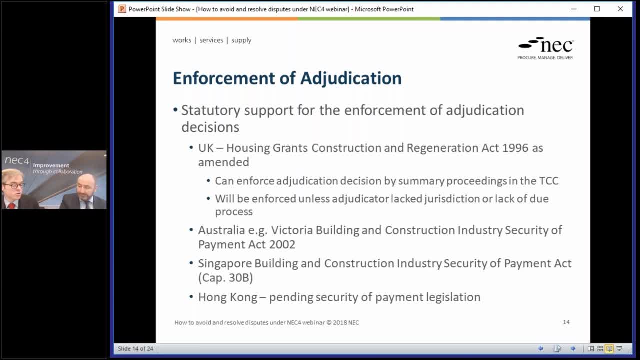 should comply with in accordance with. Yes, absolutely so. even in the countries where there isn't a straightforward enforcement in that way, a lot of countries will will be influenced by it and will and will enforce it as a contractual obligation Again and again. I guess that ultimate thing of it is binding, but not final. so there's. 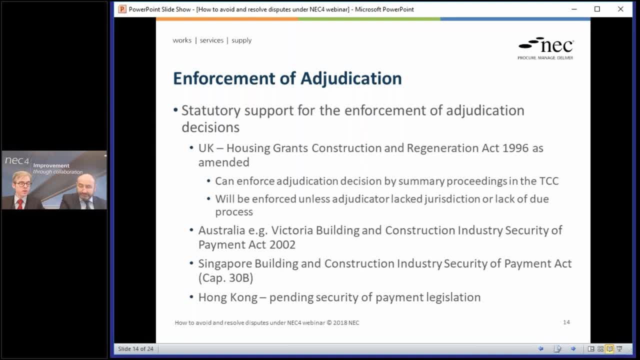 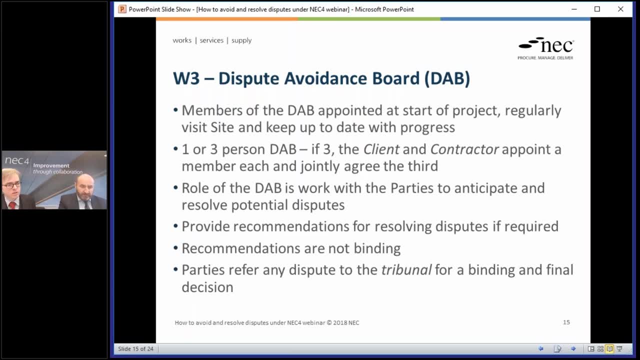 always a right of taking it to a further tribunal, Absolutely Okay. so we've touched on W1 and W2 there. I think W3 is one we need to talk about as well. I've already mentioned that W3 is specific to the ECC, and the idea behind this is to create a board that tries to work with the. 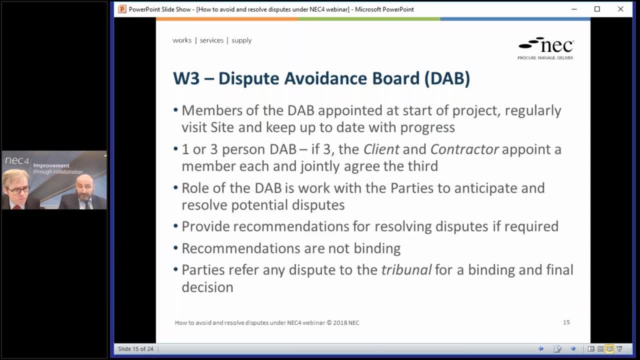 parties to resolve disputes, either- you know well- hopefully ahead of them happening, so actually being proactive, being engaged with the parties to anticipate disputes before they occur, or, if things start to become disagreements between the parties, helping them resolve it. So the members of the dispute board are appointed at the start of the project. 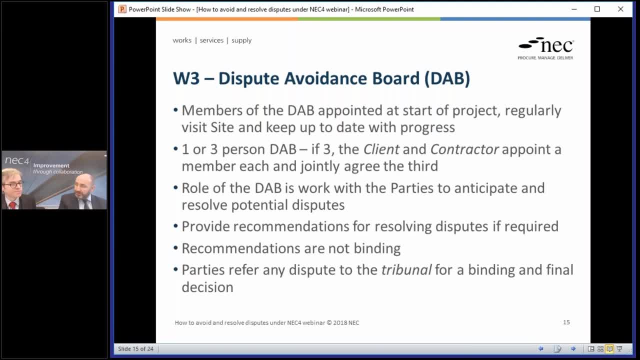 They visit site, they're involved, they get to know what's going on on the project, so they can take on this proactive function. The Dispute Avoidance Board can either be one person or three people. If it's a single person, that person is appointed by the clients. If it's three people, the client 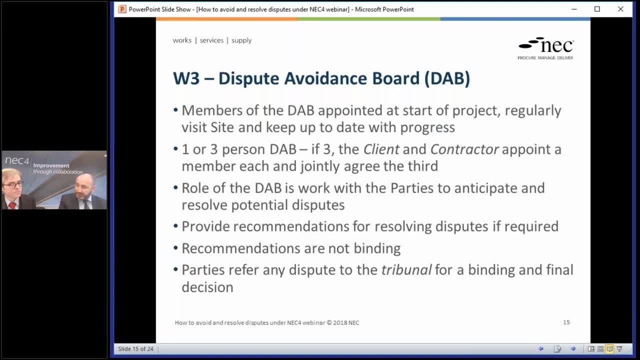 and the contractor appoints a person each and they jointly agree a third person. The key thing in terms of who is appointed as members of the DAB, it's people with the gravitas or the seniority, the respect of the parties, who are going to listen to their opinions and take on board what they suggest. So I think careful. 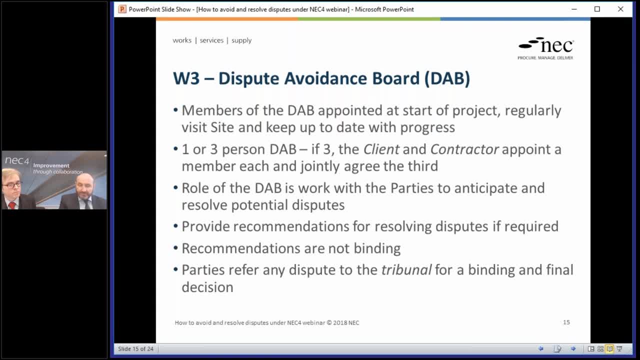 selection will be important to make this process work effectively, and one of the key things to understand here is that the Dispute Avoidance Board makes recommendations. They do not make binding decisions, so it's up to the parties to decide whether or not they will agree with that. 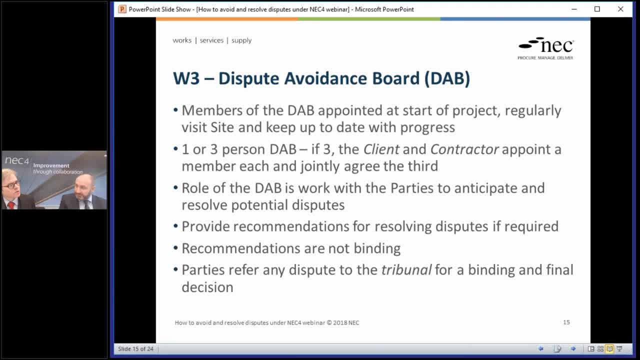 recommendation and put it into practice. They do not have to, And why would we have a dispute decision mechanism that that doesn't create a binding outcome? What would be the purpose of that? Okay, well, if the parties do want a binding decision, then they can pick W1 and they can. 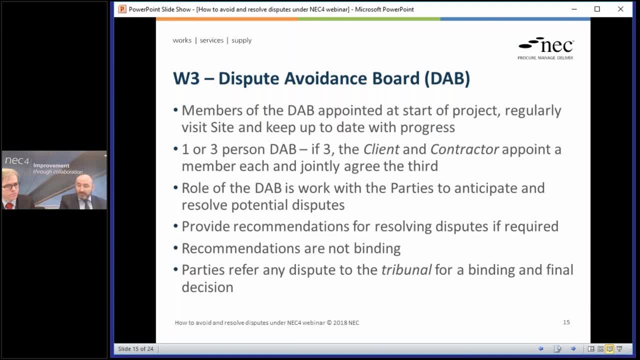 have adjudication and they can have a contractually binding decision made by a third party independent of the parties. as we've described already, The idea of the Dispute Avoidance Board is this idea that it's a much more consensual process whereby the parties are saying: let's bring in this third. 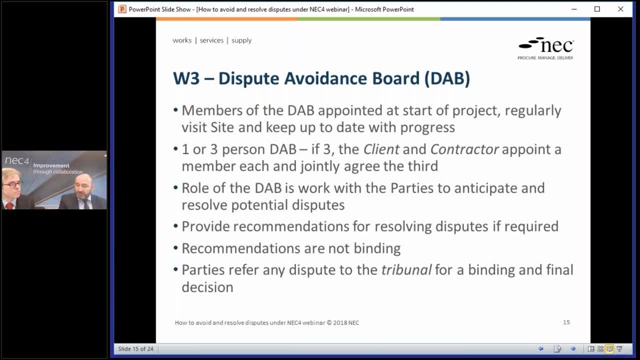 party to help us try to resolve and and diffuse disputes, almost acting in it as a quasi mediator, but also offering recommendations on how to resolve things if the parties can't be brought to the table and help to negotiate a settlement. And I suppose the fact that if you've appointed one yourself and you've been involved in the 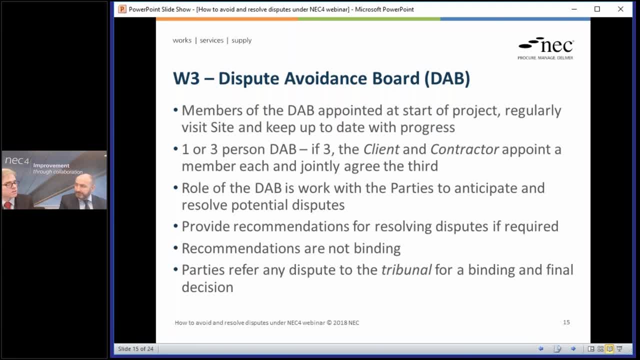 appointment of this board and you've got to know them over the project. that creates a sort of a loyalty and people would be it would be inclined to put those recommendations into effect, even without it being binding. Yeah, absolutely, and you know, hopefully these people say they are the gravitas, they are people who the parties do respect and if the the Dispute Avoidance, 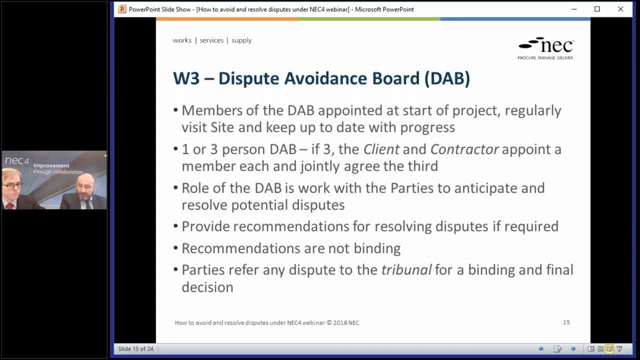 Board says: well, we think you know this is the way forward, or we would recommend, as this is the solution to the dispute, or here's how we think a tribunal may anticipate, may um may deal with it. then the parties could think, well, we can go with that, or we could ignore that and go right the way. 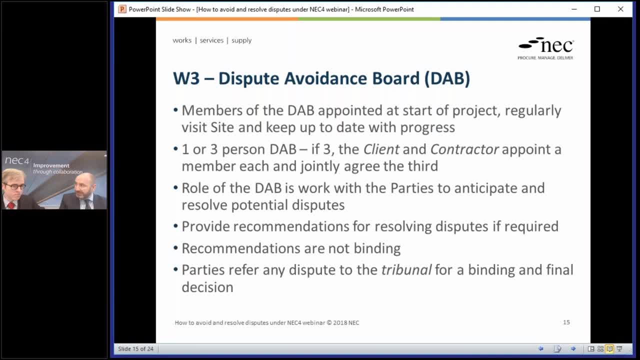 through now a formal process and a lot of time and money, but actually come back to the same point in the same place. So you know, and also another reason why not having it as a binding decision is that when you have a binding decision, you have winners and losers, and that then encourages the 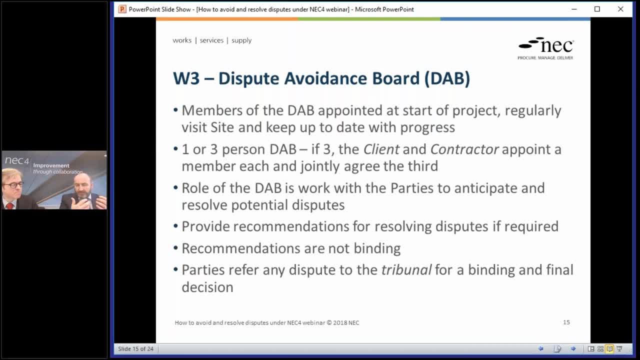 parties to maybe hold their cards closer to their chests, not to declare all their issues, all their problems and share them with the Dispute Avoidance Board, and that you may then get you know the parties trying to get lawyers or experts on their side to try and convince the board that their position is. 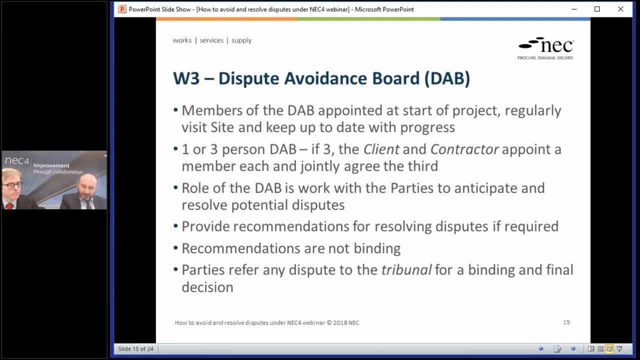 right when actually we want the board not to be bound or constrained by having to comply with. even you know. the idea is that they can maybe offer suggested commercial deals to the parties. there's almost no limit to what they can do, you know. ultimately the parties can ignore what they. 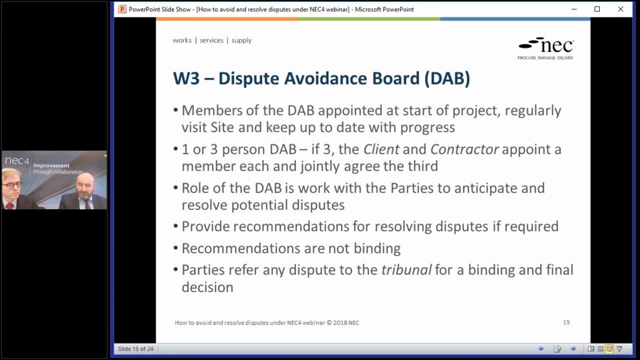 say if they feel they're going outside of their remit, Etc. but we want the board to be flexible, um, so they can have conversations, they can recommend ways forward that are going to try and help the parties resolve it. it's very much a means to an end. yeah, working with the parties to 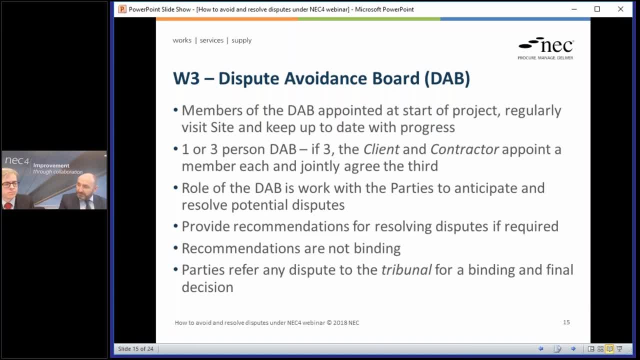 avoid the disputes rather than picking a side and picking a winner when a dispute occurs. the the DAB, it seems to be uh provoking a lot of interest. I'm seeing a lot of questions of uh arising on the DAB. there's a couple of others on senior reps, but I mean there's some 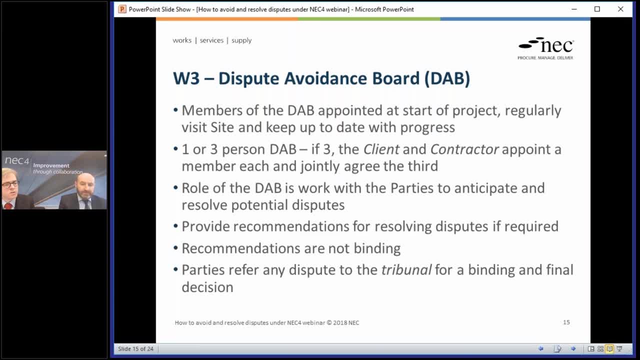 concern about the cost, uh, of the DAB and and who's going to pay for it. I mean, that's always one of the issues of you know what, you know. why should parties agree to this sort of process which is going to add cost? so yeah, under the contract, the parties would share the cost of the DAB members. 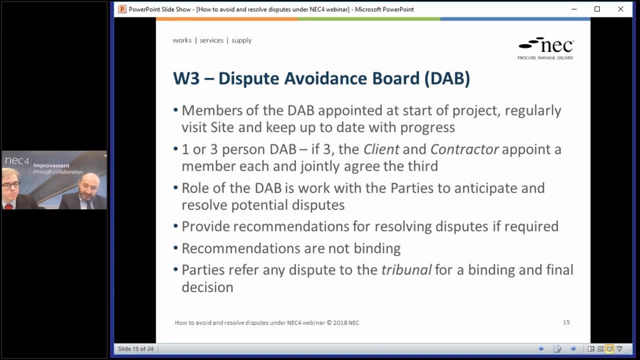 equally, and the idea being that they are both investing the cost into the DAB to avoid having to spend money on legal advice, experts, arbitrators, whatever- at a later stage, the idea being that, by investing this money, you will save money in terms of having to go. 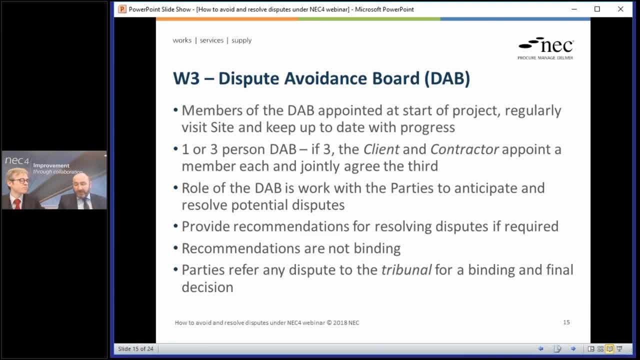 through a formal dispute resolution process. also, if the parties can stay um more collaborative through the duration of the contract, more likely to get the right result on time, Etc. yeah, and a lot of these disputes, you know you, you will have certain. in most projects you'll have certain. 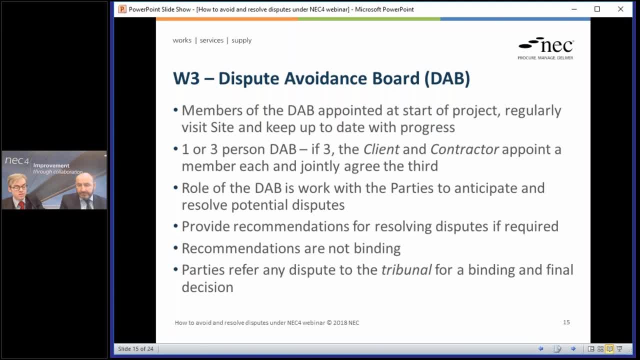 that can affect a lot of other disputes. you know as to how to assess a compensation event about. you know design, liability, these sorts of threshold points where if you get them, if you get a DAB to make a decision of principle that people can cling on to, you will avoid an awful lot of disputes down. 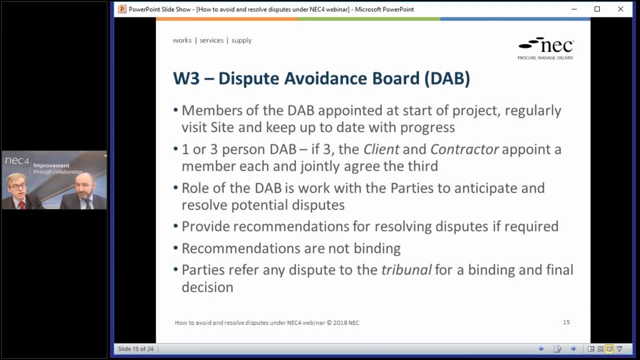 the line and that's it. so the costs really of the DAB are depending on your project, but it could be could be money well spent. so there's quite a few questions coming in on this which we'll come back to towards the end of the session, but just addressing a couple of them very quickly in. 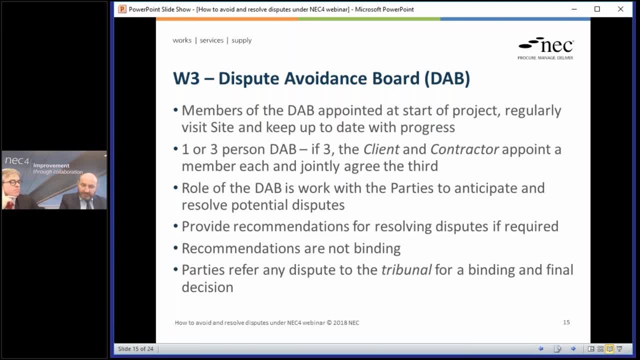 terms of the appointment of the DAB members. the idea is, if there's a one person DAB, that person is named in the contract dates of part one by the clients. if there's three, the contractor and the client would name a person each in the contract date of part one and part two respectively. and 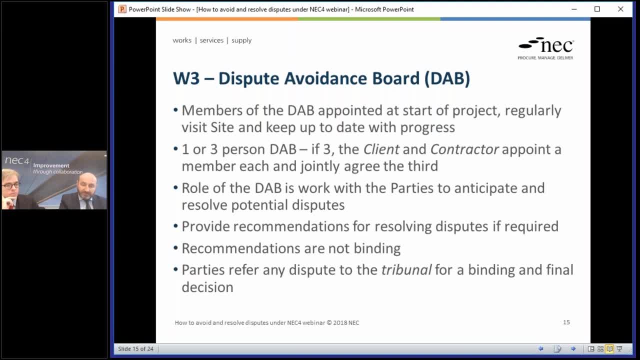 they would agree a third at the point the contract is created, and so that's how you would in effect create the DAB and have the members. the DAB can't be selected for use in the UK because it does not comply with the Housing Grants Construction Regeneration Act unless you're not doing work governed by that act. 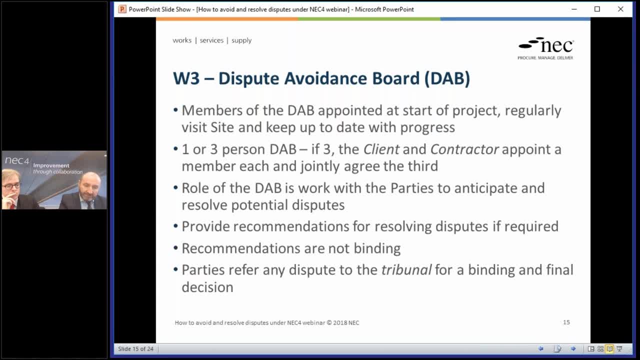 so really this is not a choice you're going to have very common in the UK for construction work. you've got W2. you have to pick that. the reason why we don't have a W2 and a W3 option to be used together is just additional cost of that. there's nothing stopping the parties creating a separate. 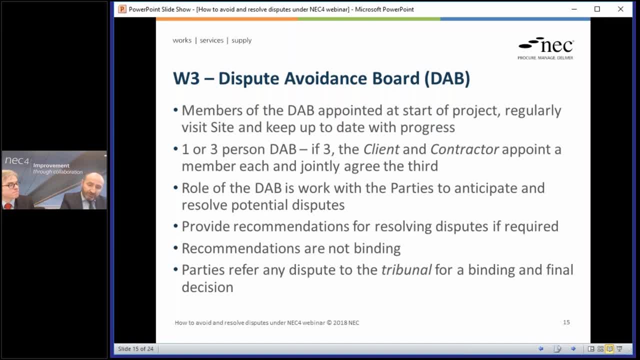 way within the Scottish ladder or having some sort of forum to hear disputes. the idea here is we have a choice of options and you pick one or the other. if you pick two, you start to double up on the same process. that's right and uh, and one of the questions that come through is about what happens. 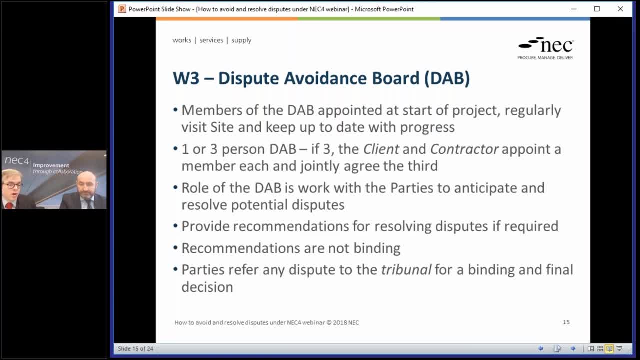 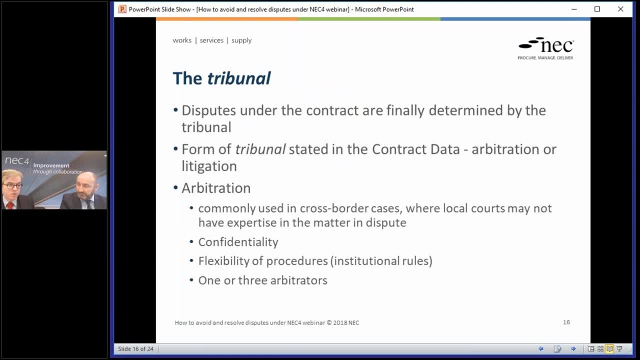 uh after the DAB? um, uh, and what happens after the DAB is, if, is, if one side doesn't like it, uh, it goes off to the tribunal. um, I mean the tribunal. when we're talking about an AC contract, it's shorthand uh for for either arbitration or litigation, and this is where you get a final determination, all of 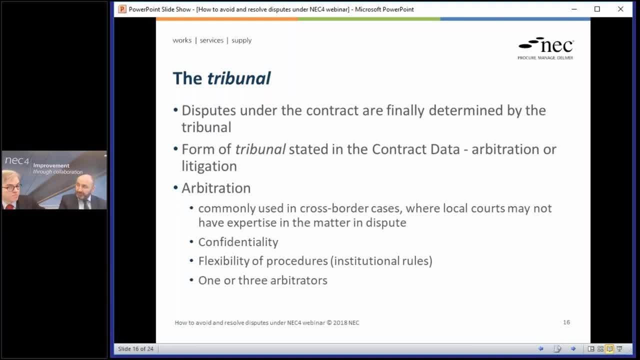 those we've been talking about. so the W1, W2, W3, in all of those, if either party is dissatisfied with the adjudicator's decision, or if they don't make a decision, or the DAB doesn't make a recommendation, or someone also doesn't like the recommendation. in all of those, your final port of call for this: 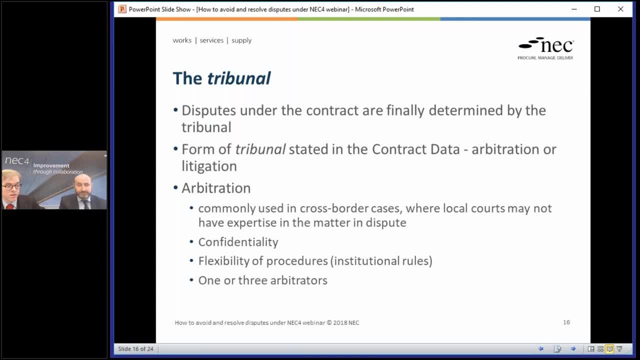 final binding decision is the tribunal, and that's right and and that you had. you should agree upfront, you should agree in in the contract data whether it's going to be litigation or whether it's going to be arbitration. um, just to run through those as options: um, in arbitration used to be very common, uh, in this country is now less so. uh, due. 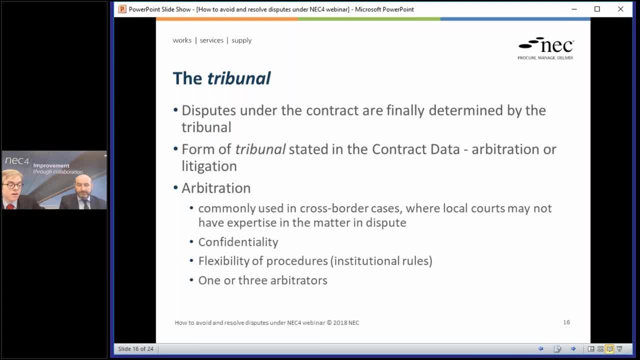 to the invention of uh adjudication and the fact that adjudication is now compulsory. um, nowadays, uh, we more commonly see arbitration in cross-border cases, international cases where you have parties from different countries on complex construction engineering cases where one side won't want to be in the courts of the other side or, as a purely pragmatic matter, the local courts might not have. 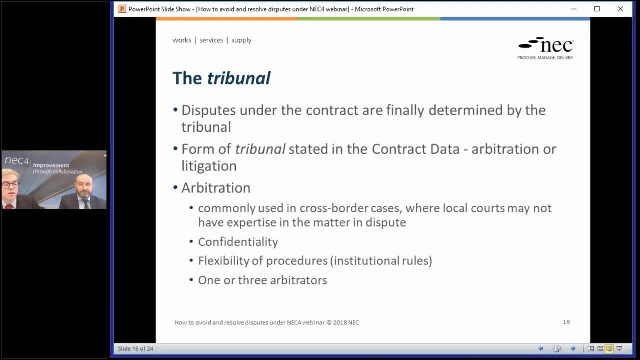 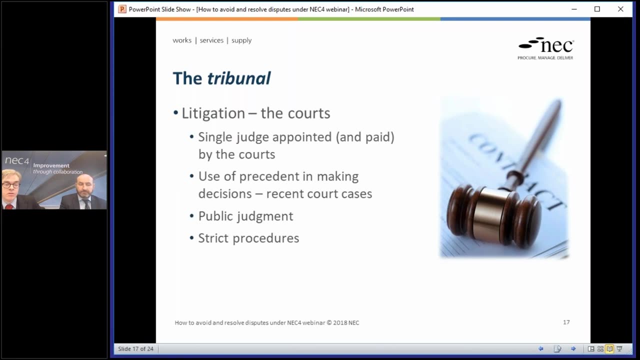 uh the expertise or the resources. here in the UK we're fortunate to have the, the TCC, the technology and construction court, that has specialist judges who only hear technology and construction cases. um and so, uh, the beauties of, uh the beauty of the court is that, uh, there's a specialist judge. 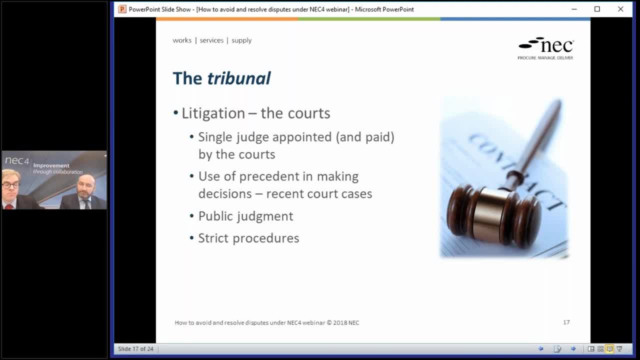 uh, you don't pay his wages? um, there's there's a solid uh body of precedent and they rely on on on the court cases, and you know exactly what you're going to do. um the the downsides possibly, um is that the judgment will be public, so all of your disputes will be known to the whole world. um, and 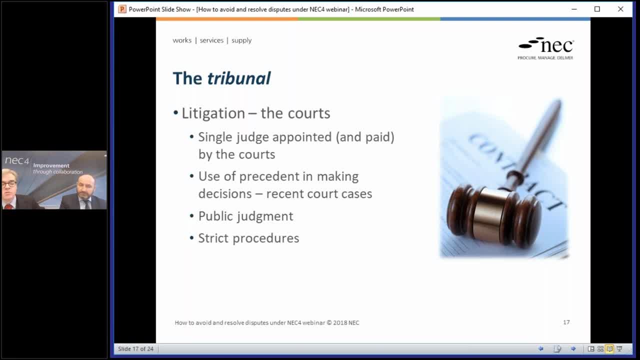 who lost will also be known to the whole world, and and civil procedure is complex, quite strict. there's disclosure of documents, uh, and it's all it. and it can be quite costly, although the courts are now taking steps to to reduce the cost and and the impact. um, 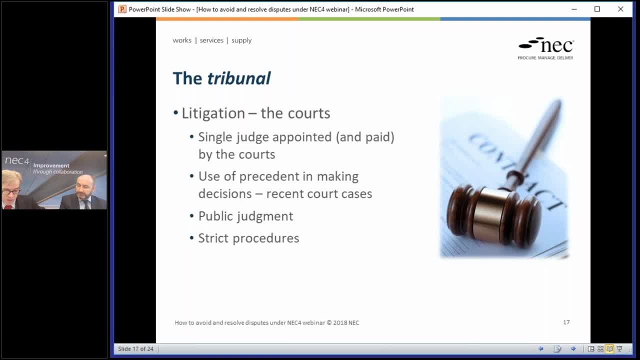 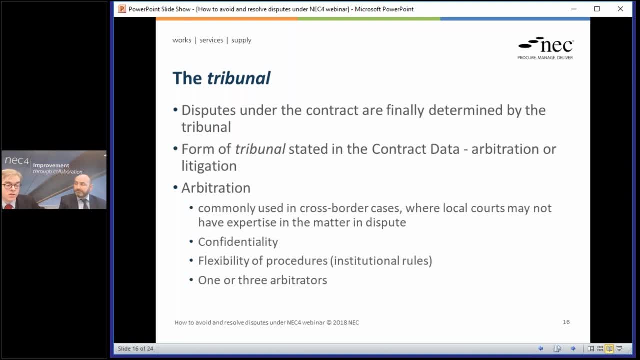 um the. the other option uh in terms of uh the tribunal is for arbitration and that has advantages um of more flexible procedures, uh that it is a confidential process. that's particularly important to a lot of clients. um, and as with the uh, as with the DAB uh option uh, there are 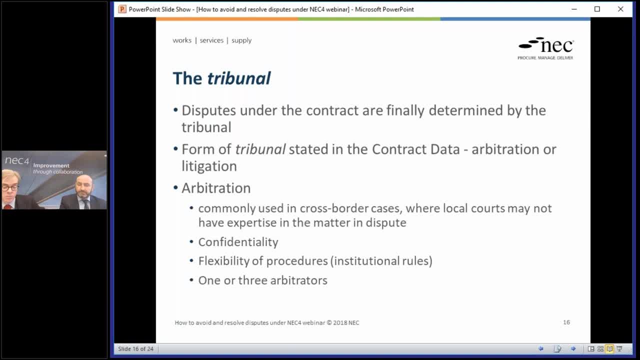 arbitrators that you can pick, uh, yourself. so either one arbitrator to be chosen by the two parties, or a panel of three. typically one party picks one, another party picks another and those two arbitrators pick the third. so the form of tribunal: you agree in your contract data and you have a choice between those two options. 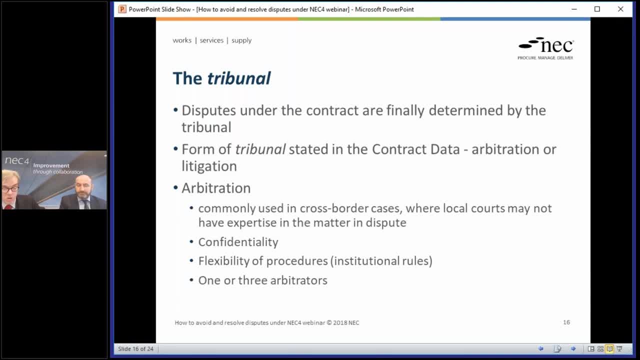 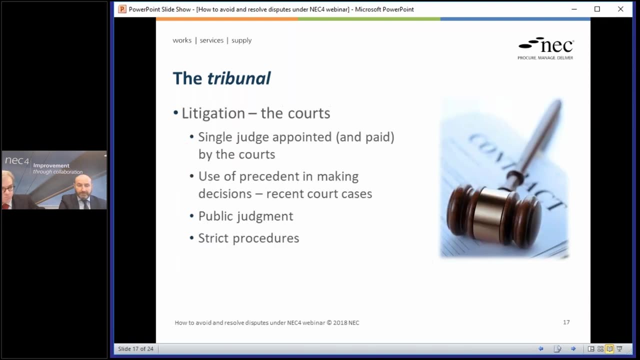 uh which present a very different format but, crucially, both of them produce uh a final uh and binding uh decision uh should either be the party be unhappy uh with any of the the non-binding, non final uh solutions in in the suite of contracts. okay, I think the last thing we have to touch on. 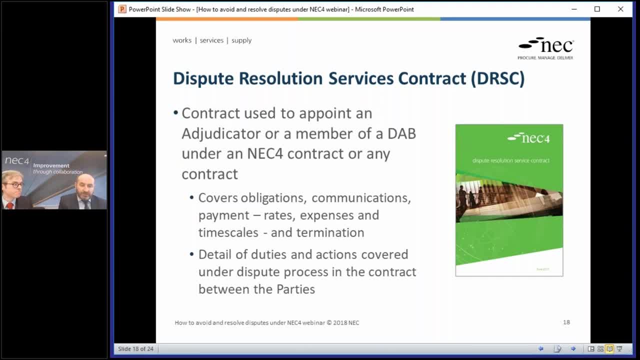 some of the questions we've received is around the district resolution services contract. so this is a new contract in the nec4 suite but, in fairness, is actually replacing and building upon the adjudicators contract which was in nec3 the reason why we've moved away from an adjudicators contract. 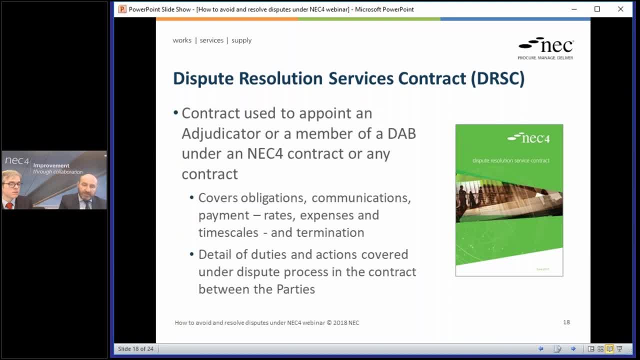 to the drsc is because this contract can be used now to not only appoint an adjudicator but also a member of a dispute avoidance board. and this contract is designed for use under the nec contracts, though in fairness, it could be used under any contract, because really, 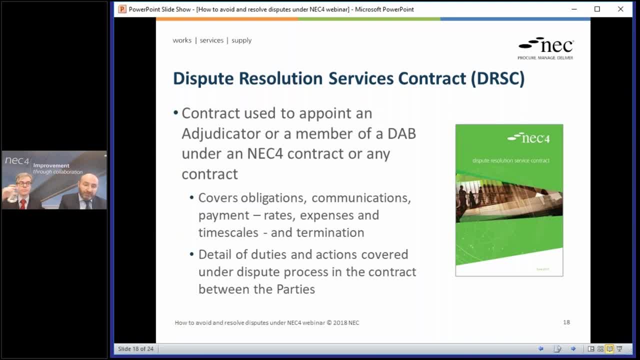 it's a contract covering the engagement of a dispute resolver. it covers the basic obligations of that person. it talks about Communications and then covers some of the key things around payments, in terms of how much they get paid, when they get paid and then, if there's a need, how that contract. 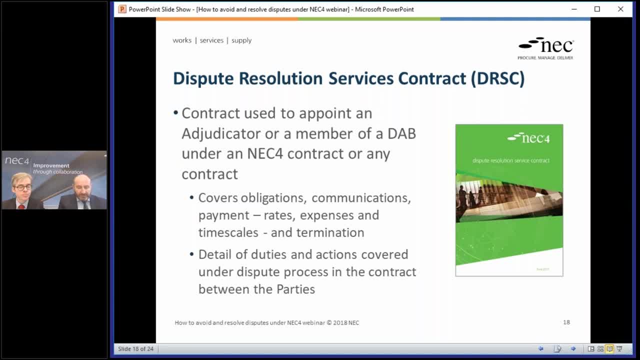 is terminated or brought to an end. so it covers very much the engagements of the district resolver. it doesn't mean what they have to do in terms of resolving the dispute, because what they do in terms of dispute resolution is determined and governed by the contract under which the dispute is occurring. 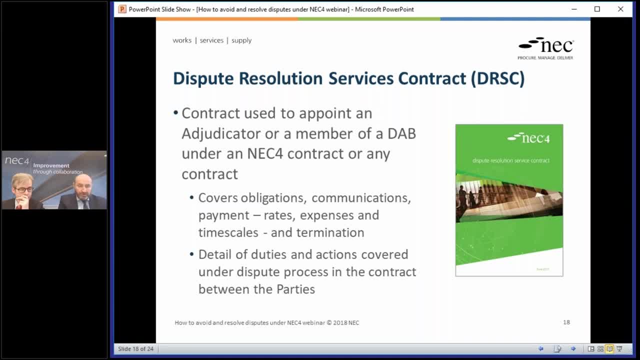 so if it's under the ECC and it's w1, w1 will give you the rules and procedures the adjudicator must follow when undertaking their duties. the same for w3 for a DAB board member. okay, so that's it in terms of the slides we had to cover. we've got a number of questions now, so 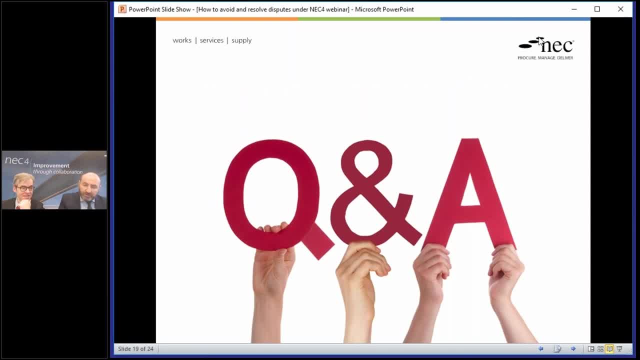 we'll just start to pick up on on some of these. um, there's a question: there is w3 option nec4 only or available for double nec3? yeah, it is new in nec4, it wasn't in nec3. I guess it could be used there. but yes, you. 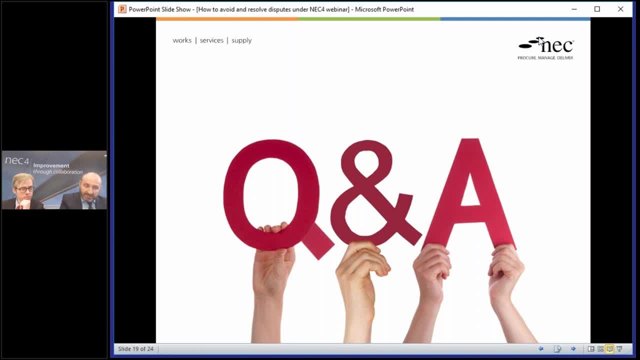 would need to do some work around changing maybe some of the clauses, adding zed clauses to give effect to it. there's another question there about the, the DAB. there's quite a lot of interest in in the the identities of uh, of the individuals, um whether they should be from independent third-party outfits or whether they can be. 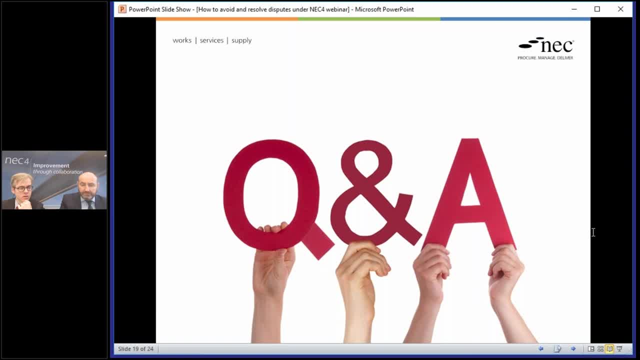 from the client or contractor organizations and that's entirely up to the parties. um yeah, I think the concept of it is that they should be external, independent entities, but I suppose it is possible to appoint DAB members, senior individuals, within the two organizations, again ideally removed from. 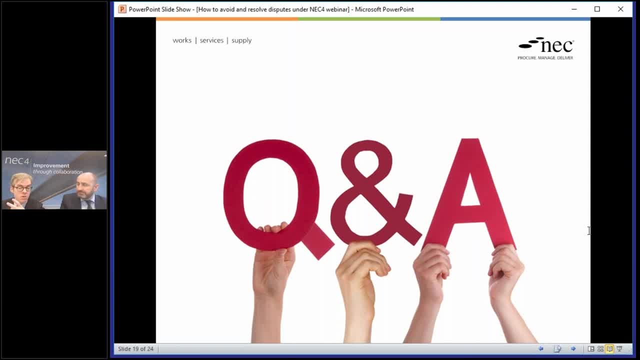 the project that that may uh it. it may create more of a dynamic that assists uh companies in in value with those decisions uh, but equally it may you know, it may cause a bit of friction with the other side when they decide that a particular DAB member is not independent. so I think the idea is: 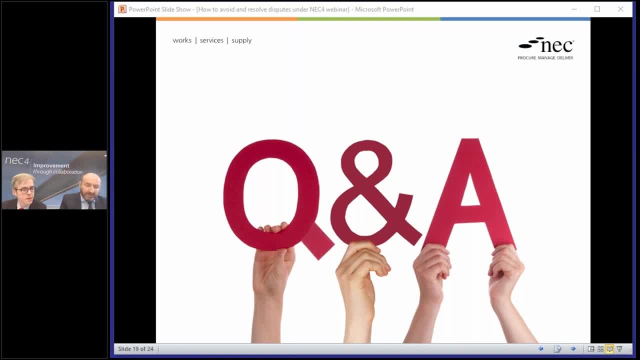 that there should be external, but there's no hard and fast rule. yeah, I think yeah. and then recommendation: they should be external to give the then the gravitas and the independence for the parties to respect what they're saying, to share their problems if one of the members is. 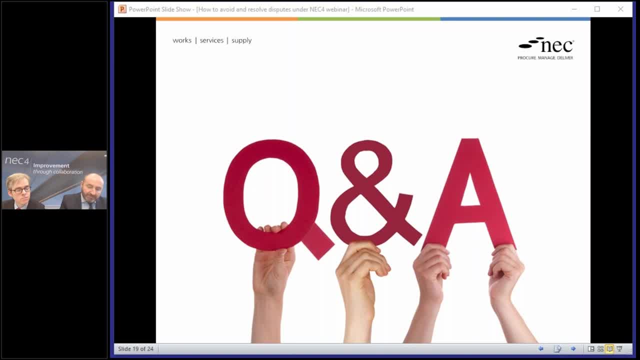 maybe from the- the opposition, if you like. if you're in a dispute type situation, then you wouldn't let anyone to share those problems with that person. it could really, I think, constrain the process, yeah and yeah, there's a there's a question about again about DAB decisions. 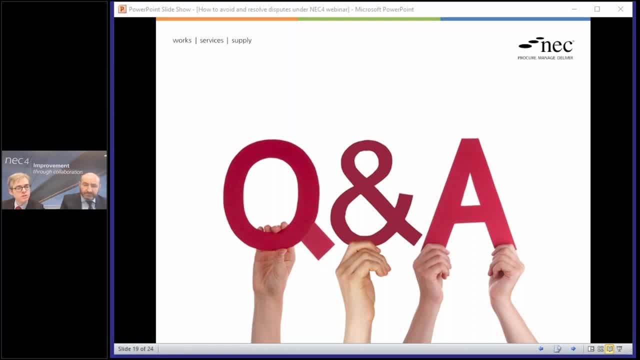 and and the challenge uh to those uh decisions and and what the grounds might be to challenge a DAB decision. I mean, I've been through that uh scenario and, in fact, what one in? in fact, one is not really challenging the DAB uh decision as such effectively when you go uh the case. I'm thinking. 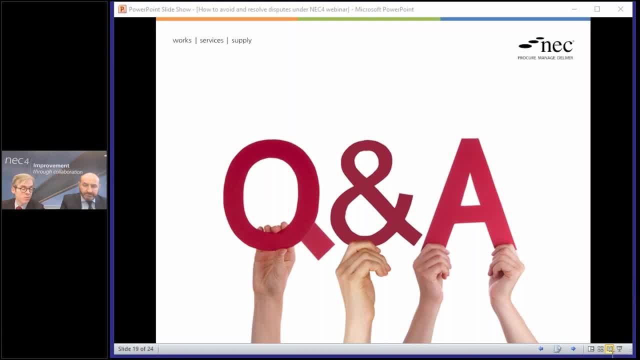 went from a DAB to arbitration, but the same thing would happen if you went from a DAB to litigation. you're not really challenging the decision as such, you're just having that dispute afresh, and the tribunal in that case did read the DAB decision but didn't have much regard to it because it knew. 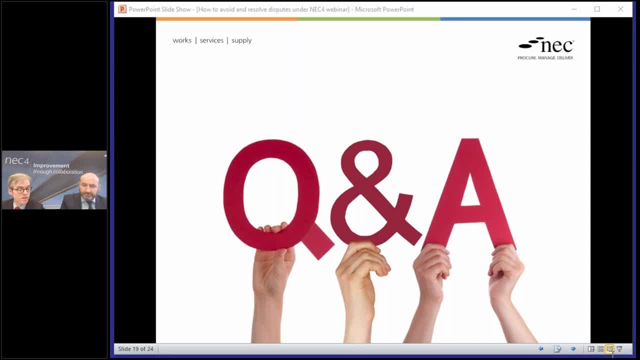 that you know, the DAB's scope was was relatively limited and they didn't apply necessarily the same tests that the tribunal would. so, um, the simple answer is that you can challenge a DAB decision under broadly any grounds you like. um, or you may prefer just to hear that dispute afresh, without regard to the DAB decision. 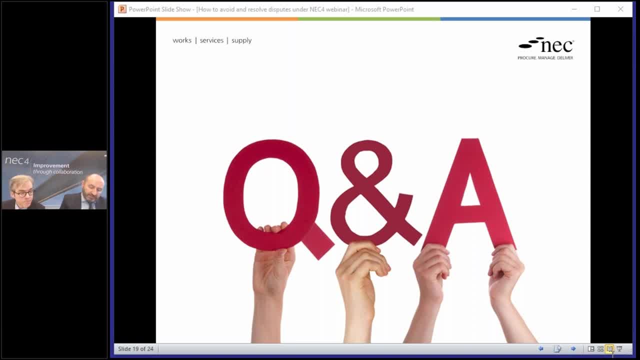 okay, another question we've got in um someone's highlighting a concern that sometimes people who are working on a project and have disagreements don't want to refer them to senior representatives because it may reflect badly on them not agreeing into the site level, which I think you know is a a 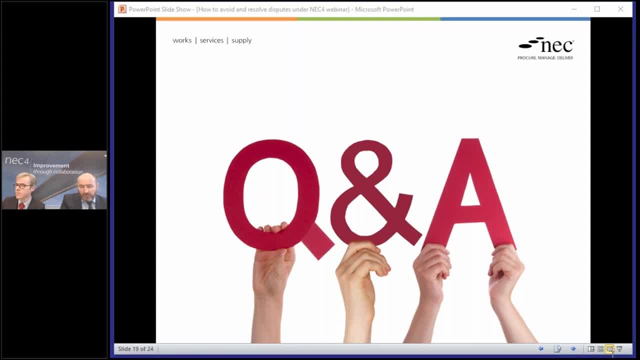 situation we can all sort of appreciate and may even have experienced. one thing we do have here, as we outlined in the talk, is that we have this final assessment process, so that would have to drive things to the senior representatives um if they were being agreed as part of that final assessment stage. now, okay, that only occurs at the 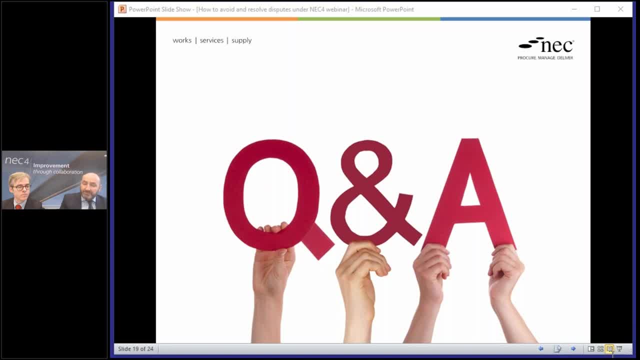 very end of the job four weeks after the defect certificate. um, I think, in terms of getting things referred more frequently for like as and when disputes actually do occur, that is going to be down to the parties. for example, managing the compensation process effectively, PMA making the contractor enforcing default acceptance of their quotations where the project manager isn't. 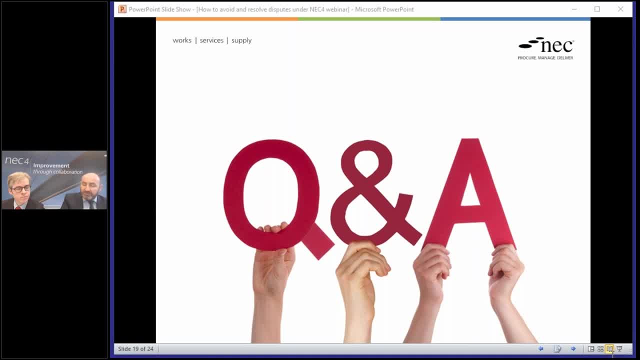 engaging. so I think there are makes to try and force issues to resolution, um, and also maybe some education of the of the teams, to make it clear that actually if they can't agree at a site level, that's not a bad thing, it's part of real life. and lifting up to senior reps is the 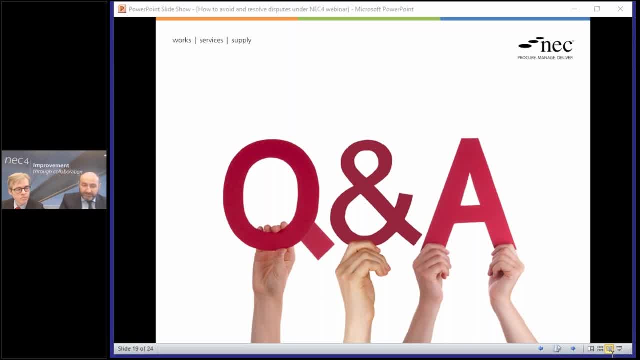 right way to go. better that than having no decision at all. um, question there about the application of housing grants: how? why does it apply? well, exactly, I mean, that is actually not a straightforward question. um, the specific example uh you raised, uh, in the question about whether a major highways. 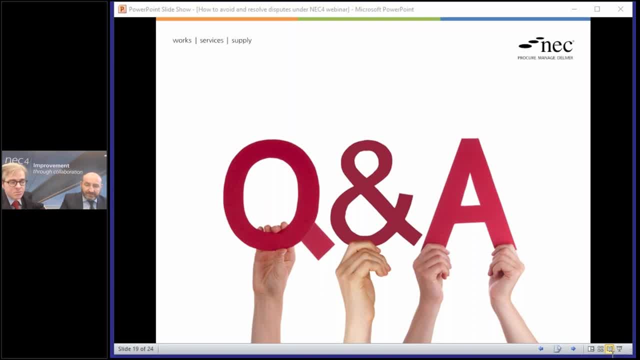 projects are covered. they certainly are. um, the core here is the concept in that act of uh, construction operations. I'm going to say section 105, but to my shame that may possibly be wrong. but anyway, there's a section that defines construction operations. long list of what. 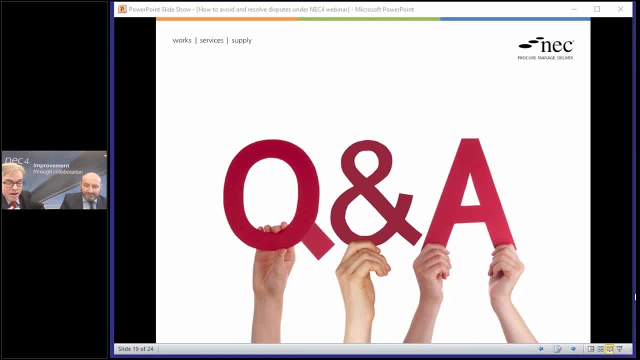 it includes, and there's a list of what it doesn't include, um, and- and you'd need to look at that in each case- there are some devilishly difficult cases which involve some construction operations and some which aren't, uh, covered by the act, and then you're really in trouble. 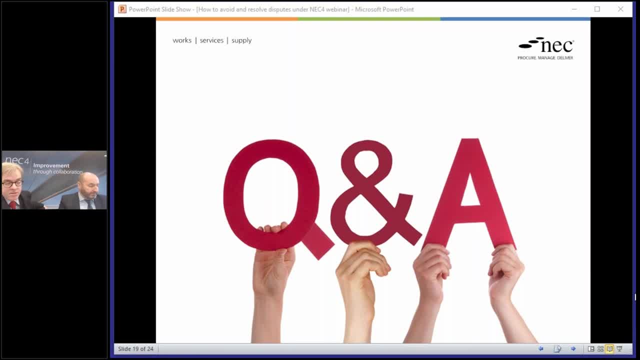 um and uh the the thing, the thing to be careful about at the outset of the project is: you know which of my, which of my packages are definitely going to be covered by construction operations- in which case I need an adjudication provision in there- and which of mine aren't, uh, in which? 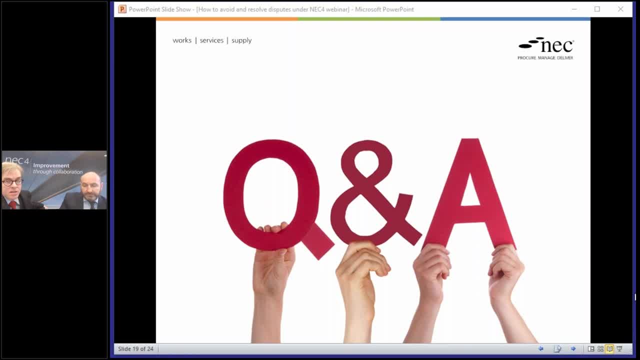 case, I can do what I like. um, so that's that's not a complete answer, but, uh, it is. it is a complex question. um, the answer is in the act. uh, but not the whole, the whole answer, because there's also case law on on that concept of construction operations. okay, um, just get some. 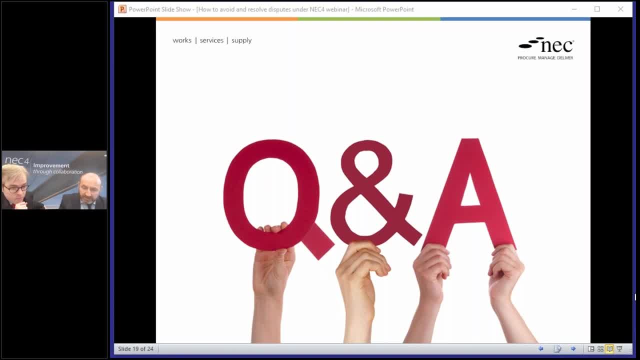 other questions, um, and we've spoken around challenges to DAP decisions. in the same way, in adjudication, decision can be challenged. you have that same mechanism and you have to challenge it, um, under clause 53, if you don't agree with it, you can't just let it stand, otherwise you. 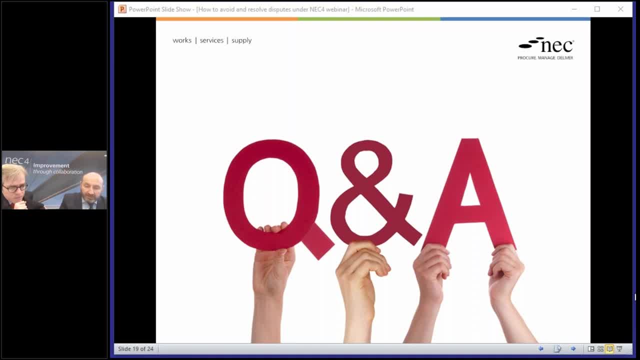 get this conclusive, conclusive agreements occurring through the silence of a party, okay, um, okay, other than, example, DAP decisions not being agreed by tribunals, the tribunals normally agree with DAP decisions. um, well, certainly, in terms of any C4 and the DAP process we have here, that hasn't. 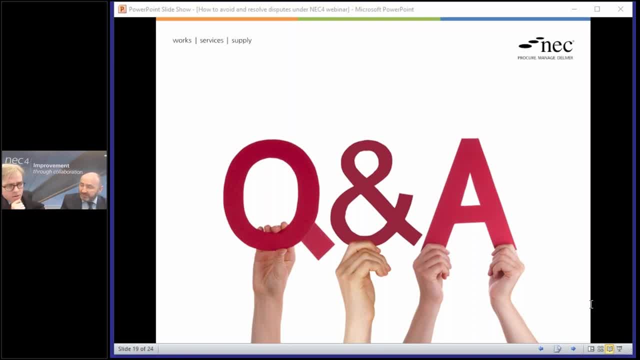 been as yet been challenged through any further tribunal, so it's difficult to answer. yeah, no, um, under the contract forms. on other contract forms, um, absolutely anything can happen. um, I I have had I have had cases where DAP decisions were overturned. this was under the FITIC suite. 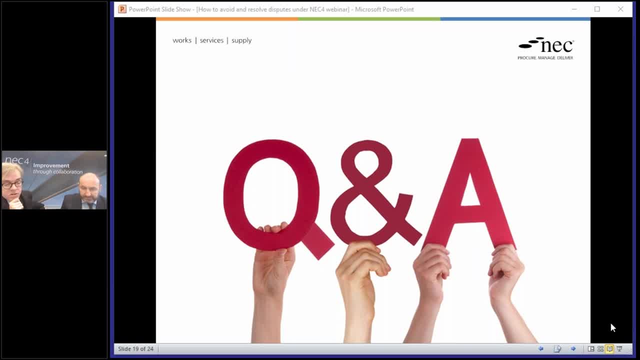 but this, the the tribunals would apply the same. uh, freedom of decision. I've I've had cases where DAP decisions were overturned. uh, I've had possibly more decisions where the decision was in the same iken fail, which is very important because I said before, uh, quite often the tribunals aren't really 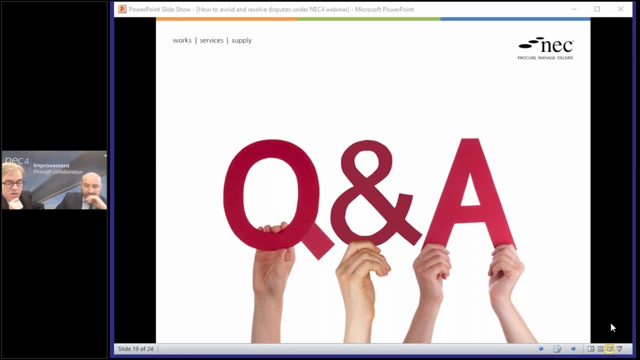 looking at the damn decision line by line and saying, well, is that the right way to do it? quite frequently they are: look, looking at the dispute, refresh, starting from scratch and deciding independently. that may be. that may result in the same decision as the DAP. it may not. 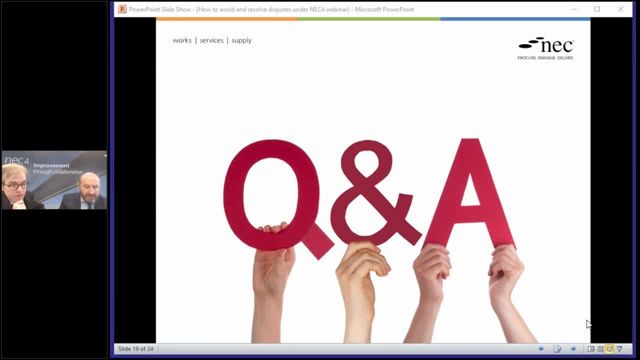 okay, there's another question that's coming around: time scales for DAP decisions and I think you know that the it's important to understand the role of the DAP and how they're meant to operate. are they visit site? when they visit site, they talk to the parties. they try to find out what's. 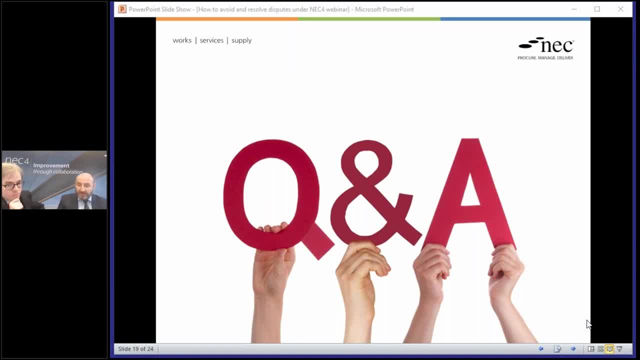 going on and they proactively try and address anything that they think could become disputes. so they can actually proactively identify things that they think the parties need to be aware of and consider a solution to, or they can deal with matters that either like refer to them as part of. 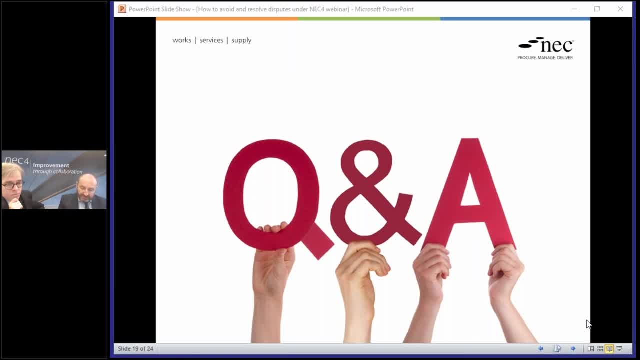 that site meeting process and also the parties can then, at the end of that process, refer to them things that they want an opinion on, and then there is no sort of I don't know there's a set time scale within the contract for that. it's more a case of the DAB working with the parties to come. 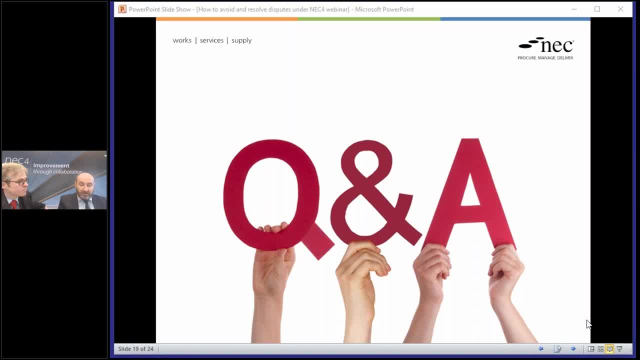 up with a, a way forward, and that may be a recommendation of getting an independent third party if it's a particular technical decision that they can't themselves give an answer to. so it may be a recommendation on a process to resolve the disputes, or it may be a recommendation. 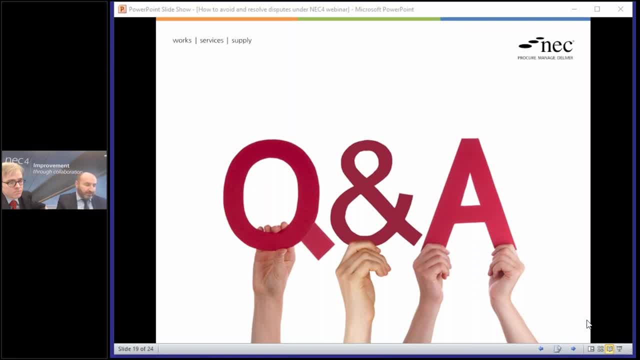 on what the answer to the dispute should be. it comes back to being sort of an inherently flexible process and very much a means to an end, the DAB working with the parties to try to get a mutual agreement. I think we're running out of time now. there was one final question I will pick up on, which is how would the panel 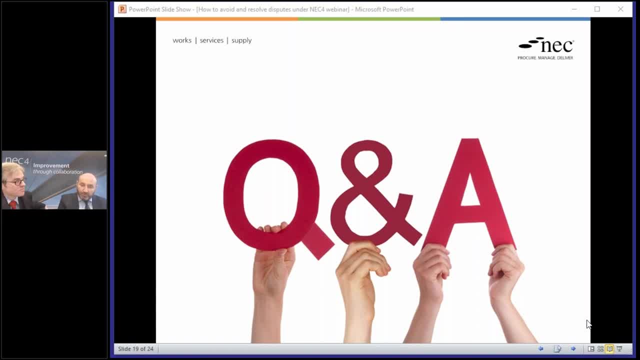 recommend the move from NEC3 to NEC4? would we recommend it and when? to make it certainly we are any spell. NEC3 will continue on. people are using it and we're going to continue on using it. there's some major projects being left under NEC3. now frameworks in place. NEC3 has a place. 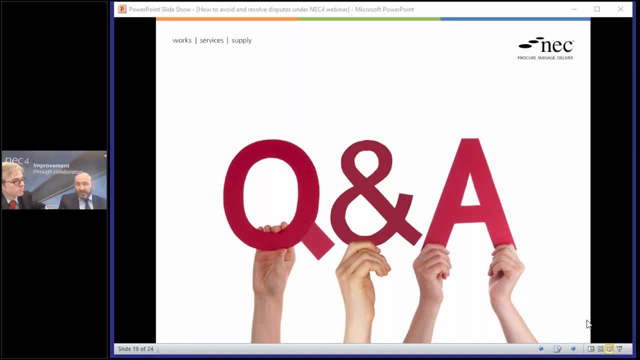 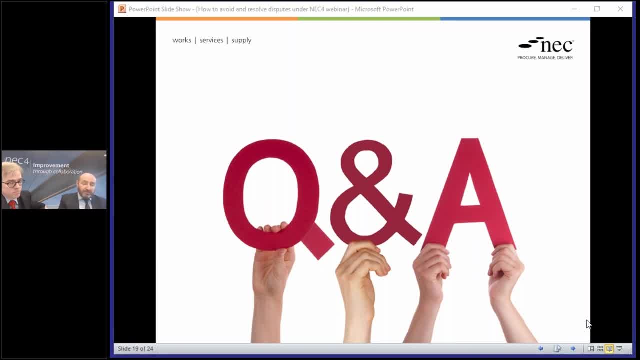 that's going to be a big part of the process. I think that's something that's going to be even more effective. I think that's something that's going to be even more effective. and remove some of the common Zed and remove some of the common Zed clauses that clients may write, however you know there is no. 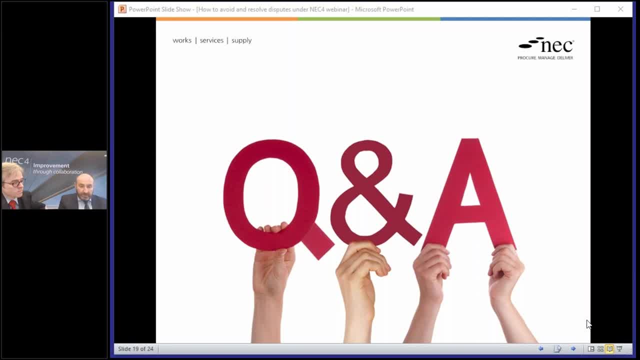 must change. there's no cut-off date for NEC3. it's when parties, I guess, feel comfortable to make that change. I think you're naturally- when new contracts come up or existing frameworks end. so I think we are unfortunately running out of time. so I thank Marcus for his contribution today. 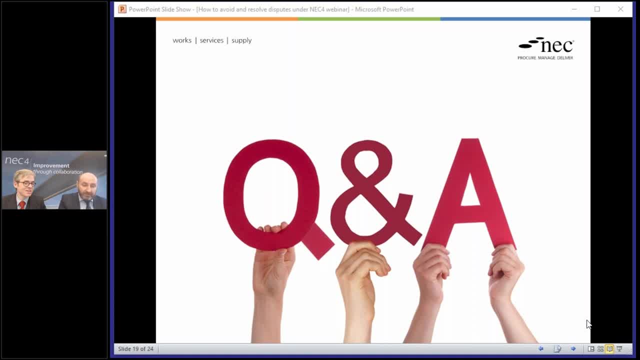 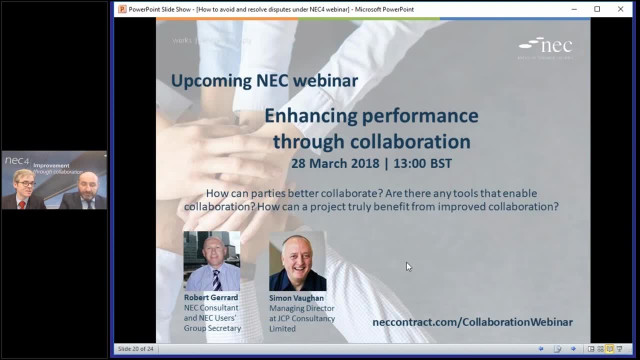 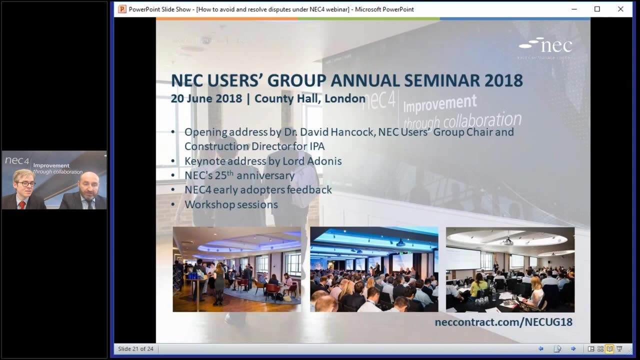 and thank you for your attendance. and just in terms of future dates for the diary to be aware of, there is another webinar coming up on the 28th of March about enhancing performance through collaboration with Roger Rob and Simon Vaughan. we then have the NEC users group annual seminar for